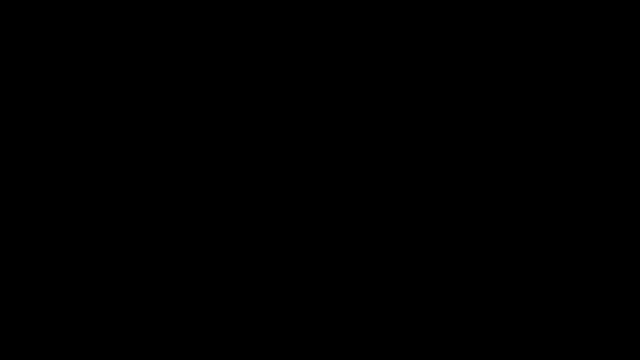 He has specialized in statistics and worked primarily with SAS, R and SPS and Excel to solve business problems, And currently he is employed with an MNC company. Good morning, sir. Over to you. You can start with the session for today, which topic is data visualization with GGPLOT webinar. 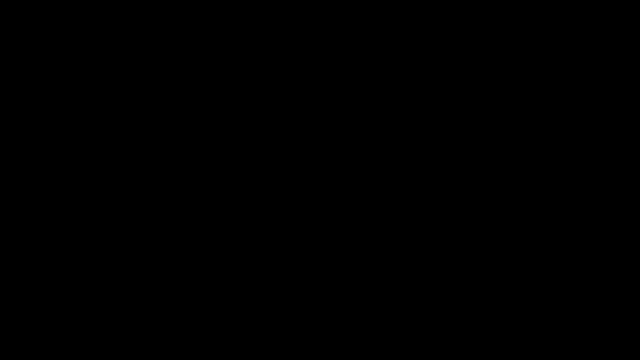 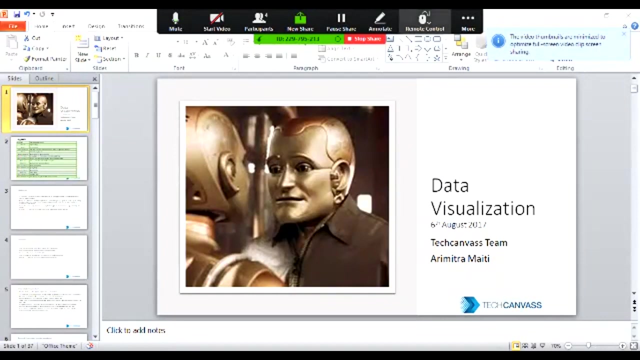 Thank you so much, sir. Thank you, Nazneen. Hi everyone, Good morning. Thank you so much for joining today, And it's really early morning on Sunday, So let me just Share the screen and let me know if all of you can see it. 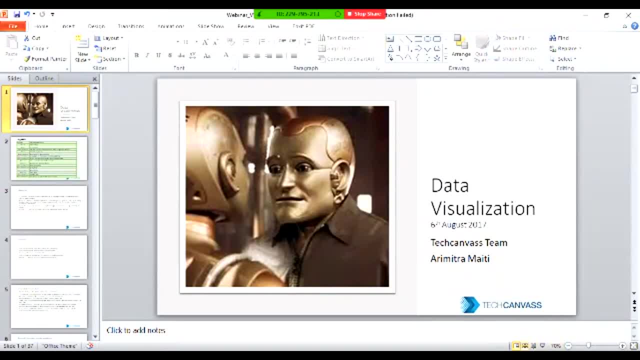 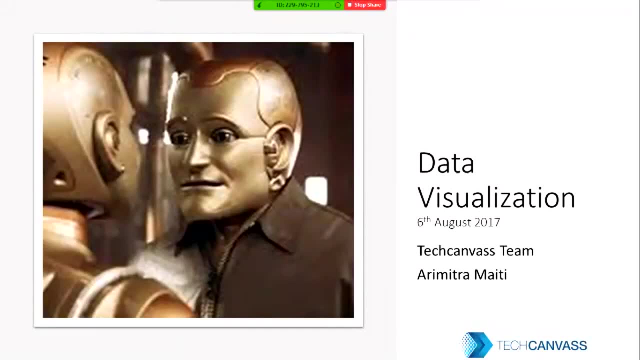 I'll just try and put it in the slideshow mode. OK, so before I start, I'll not be able to look at the chat window because I'm sharing the presentation on full screen. So if anybody has any question, please do stop me immediately so that the doubts get cleared. 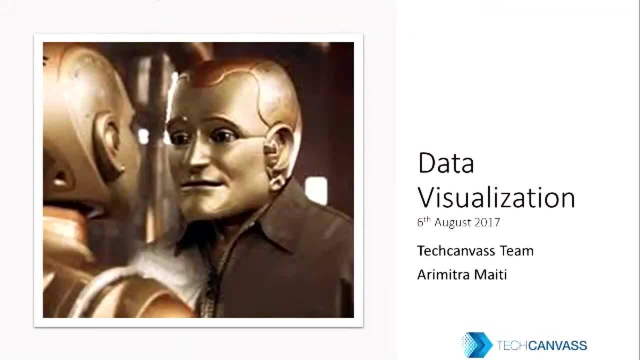 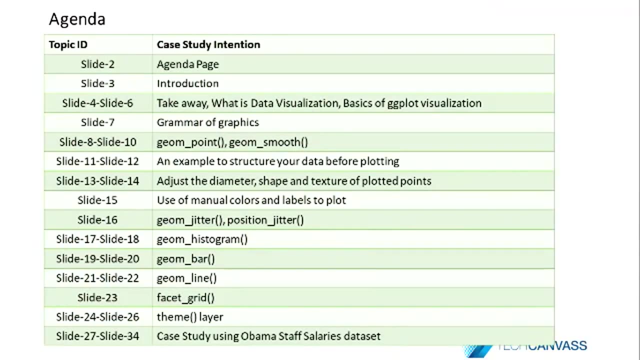 And we Uh Absorb the concepts as is, and then we make ourselves available to improvise on those concepts. OK, so this is today's agenda um that we were going to discuss today. We will start off with the start to short introduction and then a takeaway of what we want to infer from today's discussion. 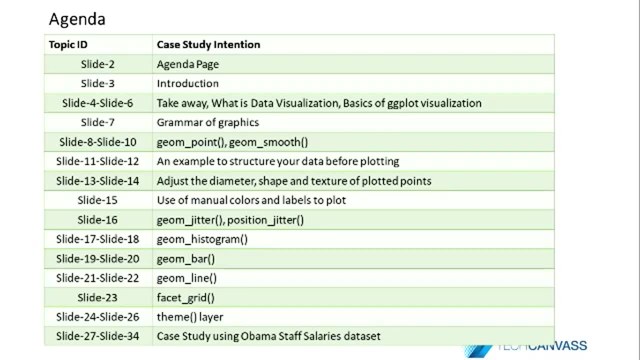 Uh, we also going to talk about what is data visualization And the basics of ggplot visualization. And from slide seven onwards, we will specifically move on to the nitty gritties of this ggplot in revolution R. And finally, from slide 27 to slide 34, which you look at the very last row of the agenda table, we will going to pick up a case study from a free available data set and see if we can use the ggplot function. 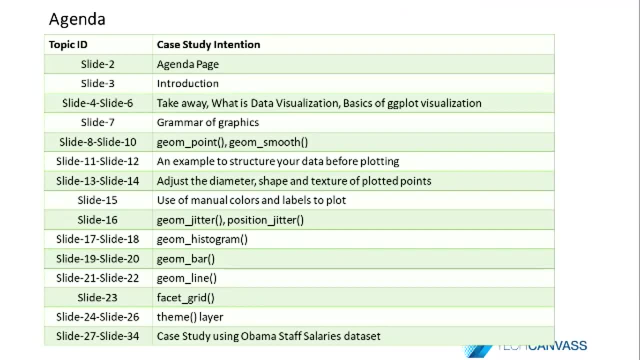 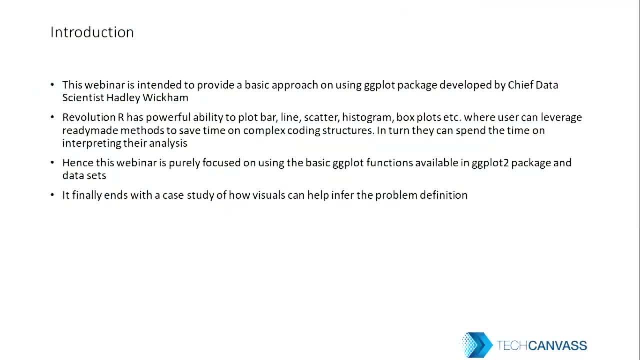 So The ggplot functions, uh, and figure out whether it helps us or not. So we can move on to the introduction here. So today's webinar is basically, you know, I I wanted to highlight the impact of data visualization on the analytics industry or on any industry where some amount of data crunching or analysis is required. 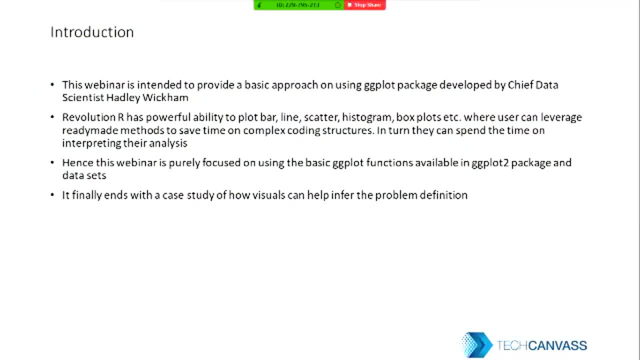 In the last slide we will talk about the difficulties that can be faced in development of data visualization. However, since we would need a tool to undergo that data visualization, I thought let's pick up revolution, R and within revolution are, of course. we have basic methods of plotting. 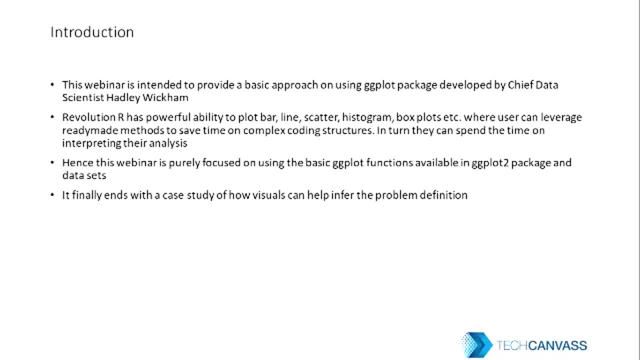 Uh, the charts, the bi charts, the box chart, box plots, the line charts. However, the chief data scientist had to wake up to has been reinventing revolutionary data, And this is in order to make our data science, uh, much more helpful for us. 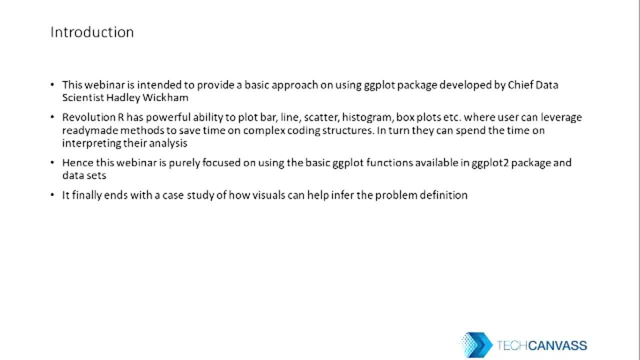 We are also going to talk about the ways in which we are going to be able to analyze the prediction of data for our data. So in this case- I'm going to start off by talking about this- We'll talk about the case study, which is a really quick one. 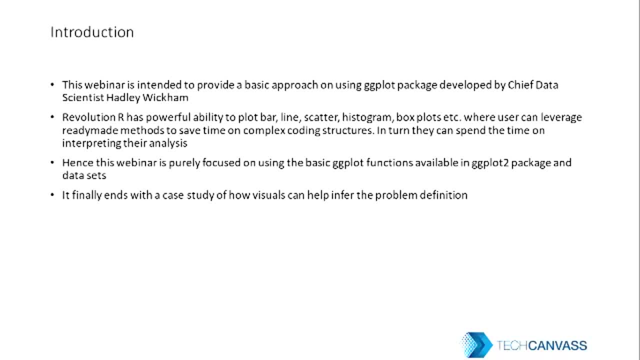 So we will talk about the evolution of data, the process of Parsley, the, the spread and the intelligence of data science revolution, R. since 2010-11, he has developed this package, which is known as ggplot. it's available once you install R. you just need to type in: install the. 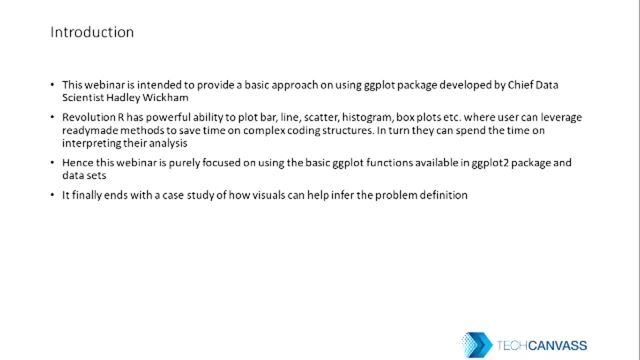 packages and then put in the package name ggplot. it will install in your directory and then you can use the library or require command to load it up. so chief scientist Hadley Wickham has been developing a lot of packages for which have been put in use today and they are widely getting used. and 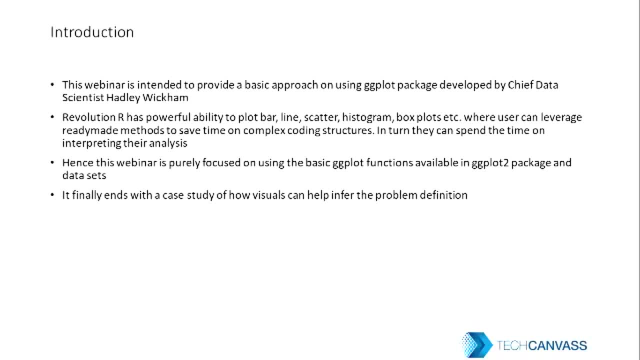 popularizing the power and the strength of revolution R. it was not like that, at least 10-12 years ago. it was a market monopoly for SAS and SPSS, but chief data scientist Hadley Wickham has introduced packages like tidy our deep lyre, lyre, ggplot. 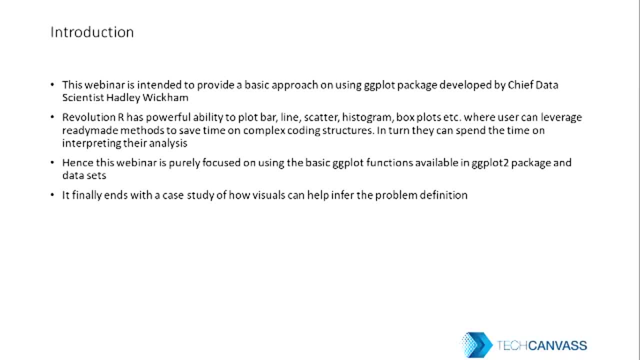 a lot of useful packages that we use today for data visualization, data extraction, manipulation and as well as statistical analysis. so in revolution R is a very powerful tool for using the data visualization realization stuff. so today's webinar will purely focus on this particular package and talk about how quickly you can leverage all the 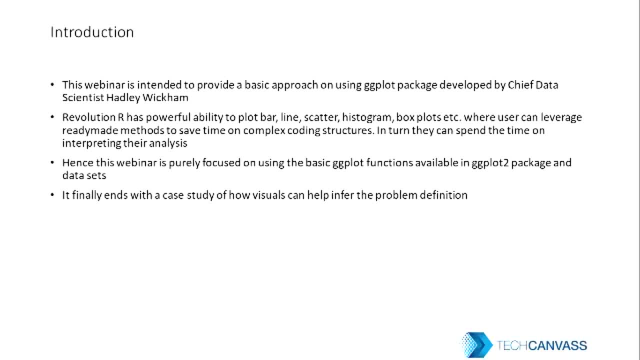 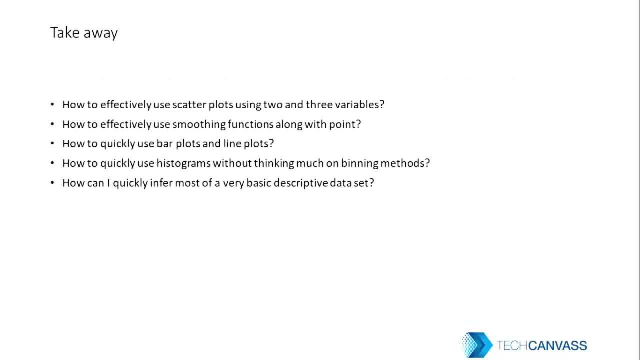 functions, of the rather most of the functions, to infer a particular business problem. okay, so what are the few things that we want to take away from today's discussion? we want to know how we can quickly use a scatter plot using two and three variables, how to effectively use the smoothing functions along the point. 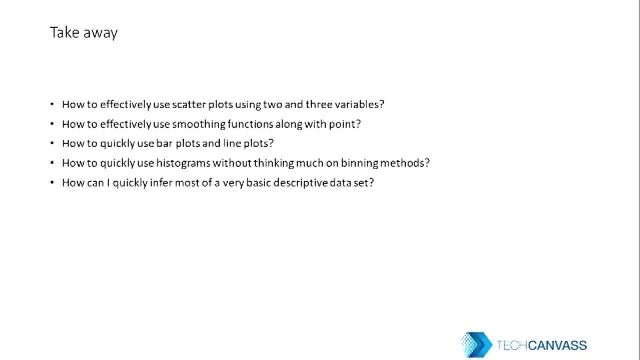 function, how we can use normal bar plot line plot histograms, what exactly we have in the binning method and how quickly I can apply those methods in the form of particular case study. not necessarily predictive but descriptive, would be fair enough to understand the power of data visualization once we can. 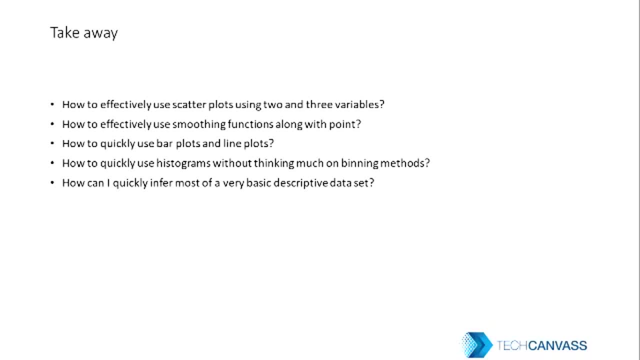 structure what we want to do. obviously, we can take most of the inferences out of that data set, so I would request, if anybody is not speaking, to go on mute, because there is a lot of background noise which may affect others to understand what exactly is going on and also the 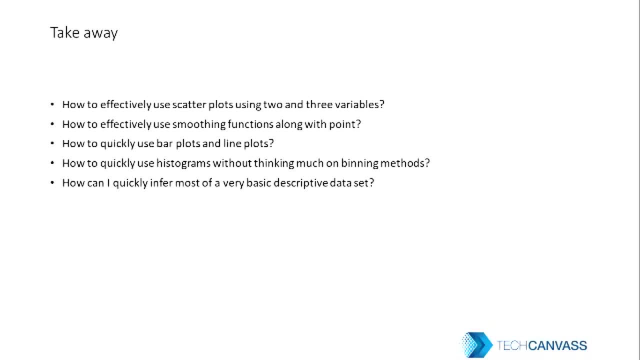 voice modulation would be a little different. so thank you for understanding and your cooperation. this is a brief takeaway of what we can take from today's discussion, but again, if you have any question at any point of time, please do unmute yourself and please let us know the questions. it will not only. 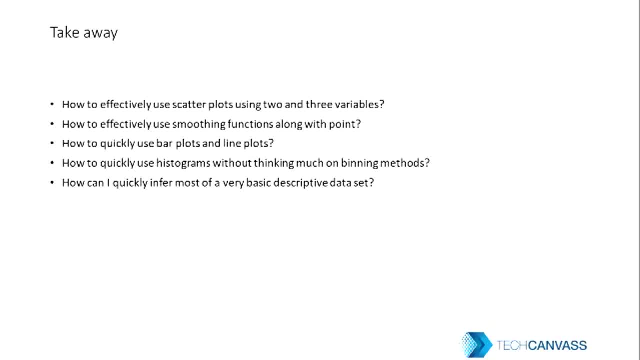 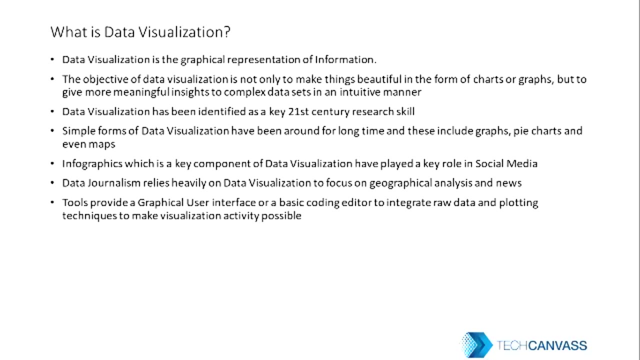 help you once you get the answer. it will help the entire audience today and it can help me as well to understand more on the concepts. so I'll quickly move on. what exactly is data visualization? this is so. data is something which is a set of, you know, numbers or text or some. 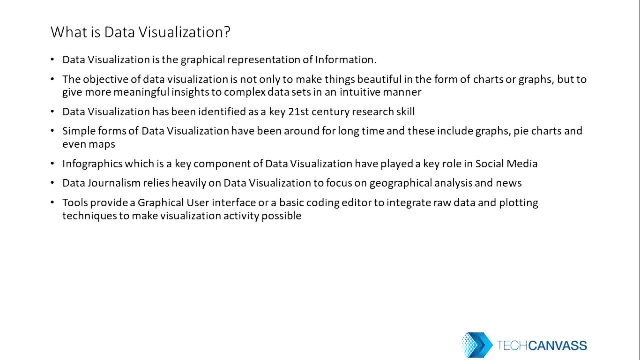 records that gets recorded in a particular platform. it can be an excel sheet, it can be a data frame, it can be a data set, it can be a table, it can be an SQL architecture. so we know already about data, but what exactly is visualization? so let's go back to our school days, when 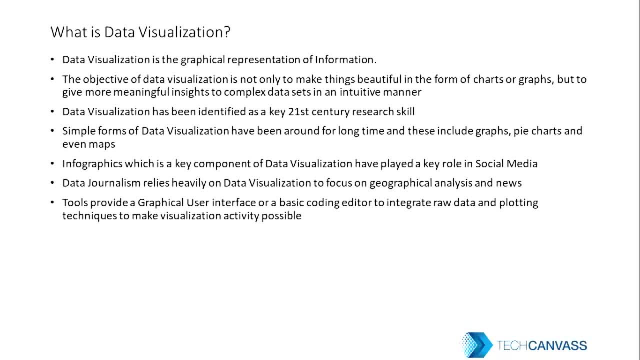 we used to read the books in any subject, so I don't recollect a book which has not been put together without a picture. so every chapter I recollect them, and not necessarily line by line. but I don't recollect a subject which used to talk about a particular concept without a picture, not. 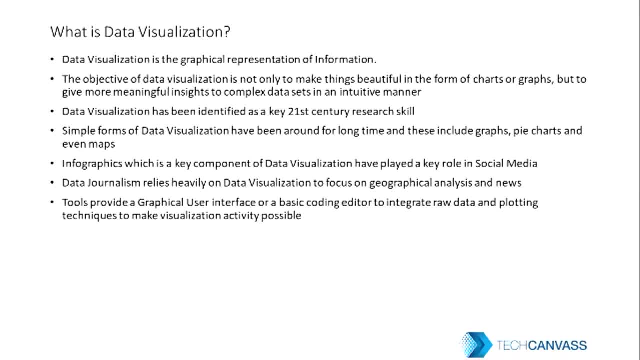 every concept line by line, but the overall view definitely used to get depicted by a picture. so people believe, or human believe, that visual memory is more powerful than a reading memory or something which you know on your own- okay, because eyes can remember more than your what you would you write on a piece. 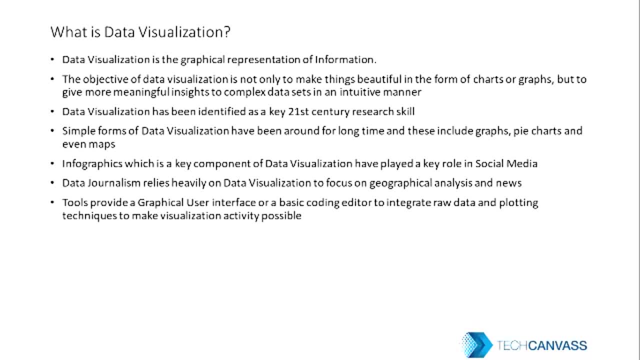 of paper. so back in our school days we used to use a lot of graph paper to you draw the line charts, to draw the frequency charts, or we used to do a lot of diagrams in any kind of subject, be it physics, be it biology, or even in. 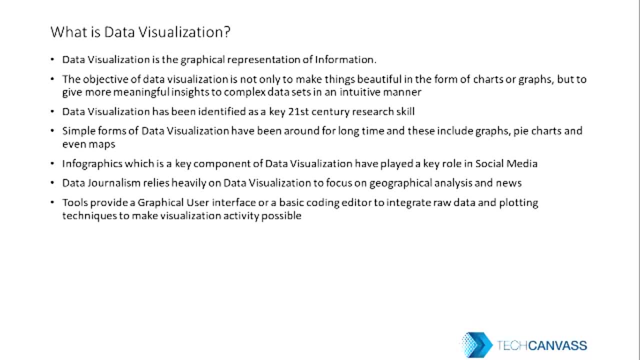 geography. we used to make a topography sheet where we used to make a short distance map of a stuff which we choose to use a dimensional scaling, I remember. so that that's all part of visualization. basically, the whole intent of talking about this is visualization is nothing new in our life. 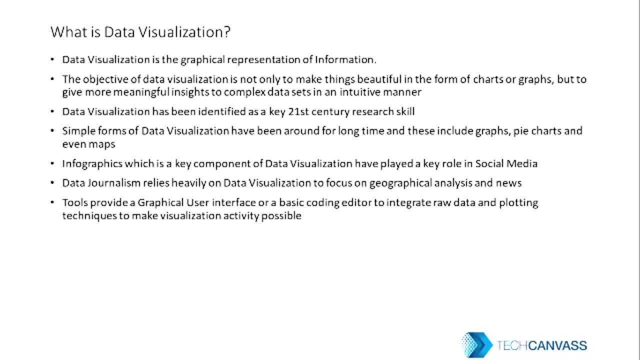 visualization is nothing new in the IT industry, or in the analytics industry, or in the corporate business or in any business. to talk about every business, use visualization. without visualization, humans cannot work. it's. the only difference is, as we go on, as we move on, there are different tools that we get to. 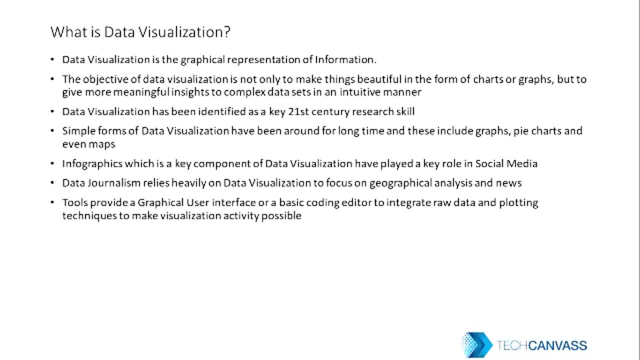 we need to know how you we need to use those tools and how we need to interpret our ideas, that we know that we have been reading till now, how we need to, you know, communicate through that language, put our thoughts into that language and make sure that language gives us back that same visualization. we. 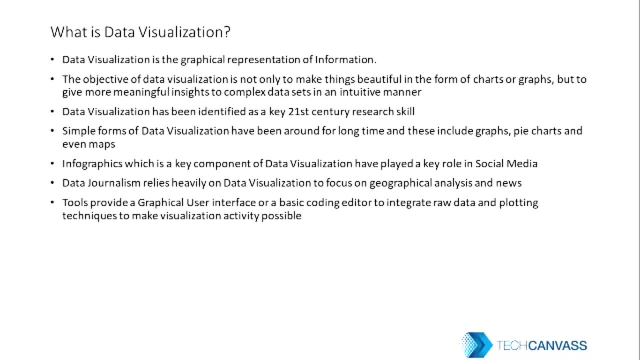 are dreaming in our minds. that's all I know. some somebody might have done that visualization in visual basic. somebody might have done it in plain Microsoft Excel. somebody might have done in PowerPoint. which we are doing today again is a part of visualization. so it is. it is nothing new. so visualization has. 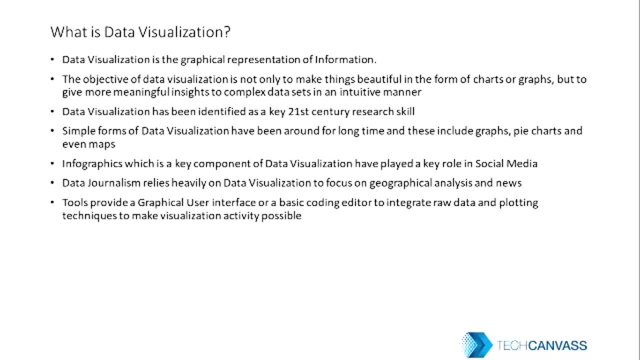 been a key member in all different industries, especially social media, especially politics, especially any kind of business, major driving business in the world that gets drive driven rather by visualization. okay, so I won't go line by line on these. you know traditional definition, but what I wanted to give an essence to the audience today that don't take a. 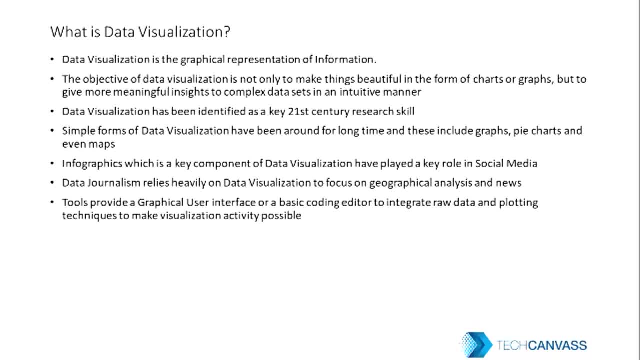 back step of while hearing the word data visualization. please don't take a back step while you hear about tableau, clickview or revolution. are these things are nothing but a language that we need to speak, that we know how we need to speak, and once we know how we need to speak, why we need to speak, one thing we 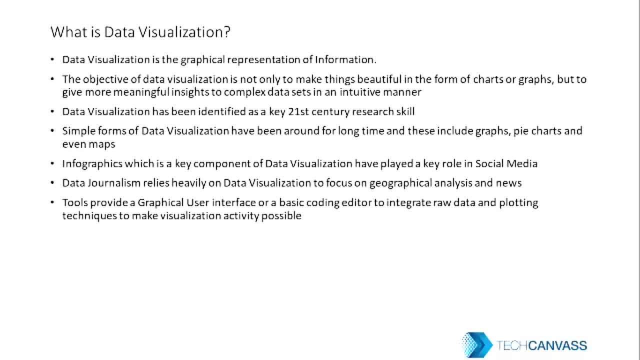 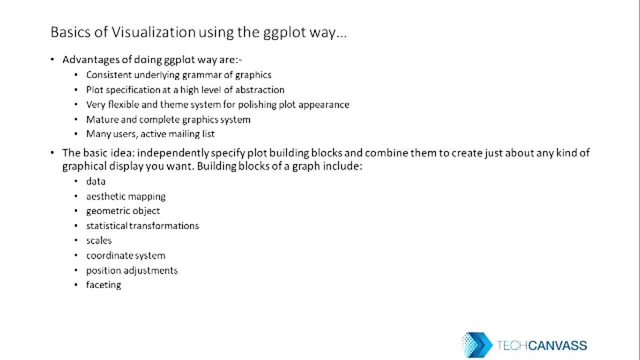 can be sure of is that our language needs to be communicated in a way. if it gets communicated in a proper way, the other end will throw us back. what we are planning in our brain, what we are planning to do, that's all. it's just a medium of communicating with the computer. okay, so quickly, what exactly is? 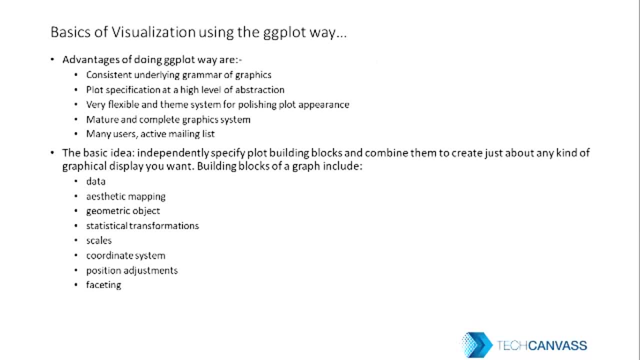 visualization using the ggplot way. now quickly talking about the advantages. apart from the basic plotting methods that ar has, ggplot uses a consistent, you know, underlying, grammar of graphics. now, what exactly grammar of graphics? we will talk about that very shortly. it has got different layers on. 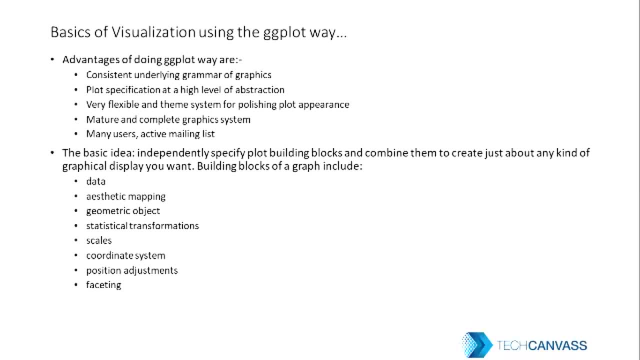 which this entire ggplot packet is distributed into. we can plot specific things at a very high level of extraction, very flexible team system- mature and complete graphic system- mature. Many users have been using it for a very, very long time since its evolution And it can also be, you know, fed as an active mailing list. 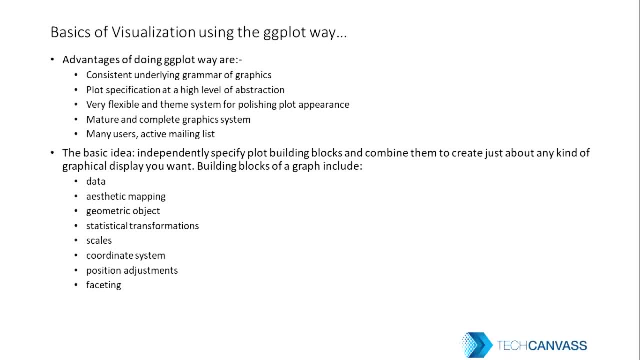 where you can directly create the charts and mail it to the users, Just like other tools. this is a very common functionality which SAS has. The basic idea of ggplot is, you know, independent. It's independent of any work that you do in R okay. 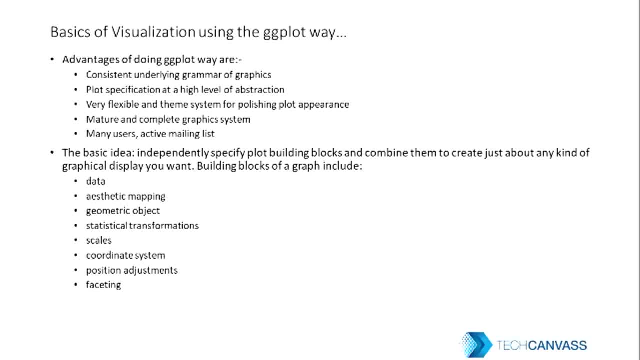 When R got invented by the scientists of New Zealand, they created certain functions which cannot be modified. okay, The outputs that were coming out of Revolution R, those were pictures which cannot be modified. Now Hadley-Wickham created this package: ggplot. 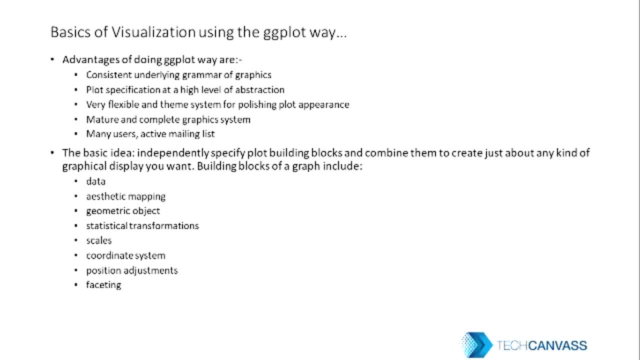 which allowed It allows users to create plots as an object. You can modify that object and do whatever you need to do at your subsequent steps and make sure you can keep on modifying them until you are satisfied, which you cannot do in R basic plotting functions. okay, 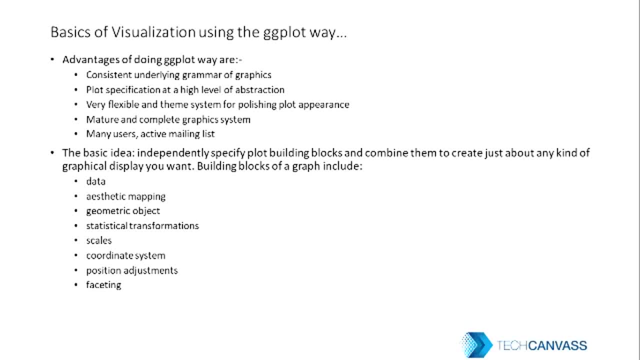 So this is one of the biggest advantages which ggplot provides compared to other packages, And this is one of the This is one of the most driving feature of ggplot, because of which it makes available in such a great scale of use to the users. okay, 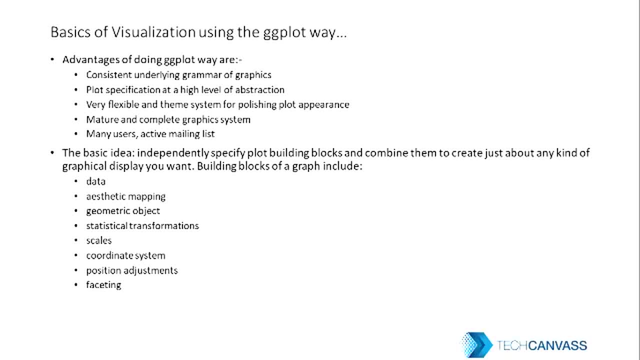 Unless you are able to modify those plotting functions or those work that you are, Those coding little bits and pieces of coding that you're doing. if you cannot modify them, it's of no use. You have to write that all long piece of code until you're satisfied. 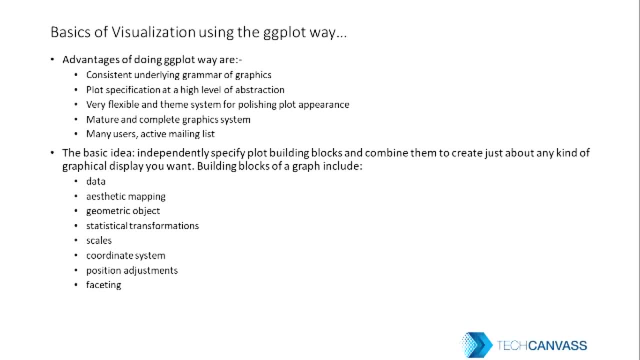 Remember everything in your brain and the output comes out as a picture. That becomes really difficult. So ggplot2 addresses that difficulty and allows users to create and modify charts, labels, backgrounds, everything, even statistics. within the chart as an object, You can modify each and everything. 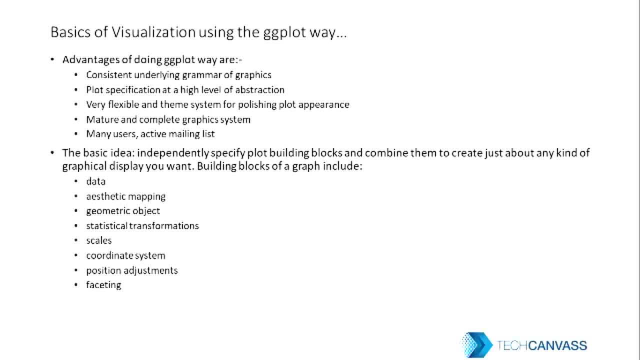 until you are satisfied. So there are different building blocks of ggplot2.. First, you need to feed in the data You need to know about. What is aesthetics? What is the geometry in ggplot2?? What are the statistical transformations? 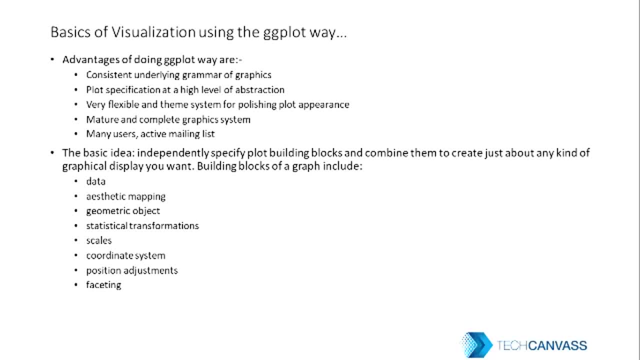 How do you modify the scales, the coordinate systems, the position adjustments, the face setting? These are very technical terms. All of this, or rather most of this. We have a time limitation as well. Most of this have been addressed in the PowerPoint. 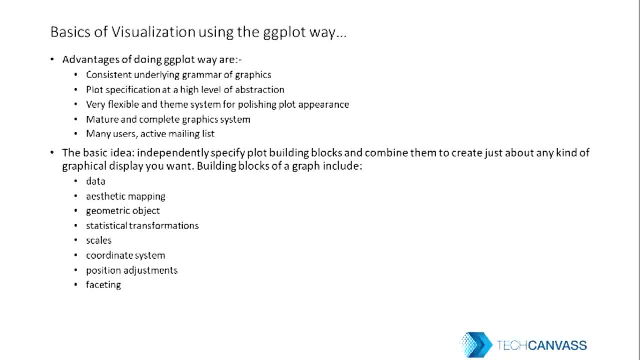 However, if you think there are, Most of the very common things have been fed into this presentation, but, however, this is not complete. I really, really encourage you to go and search the facts on the internet, Do it yourself, Practice it after the webinar. 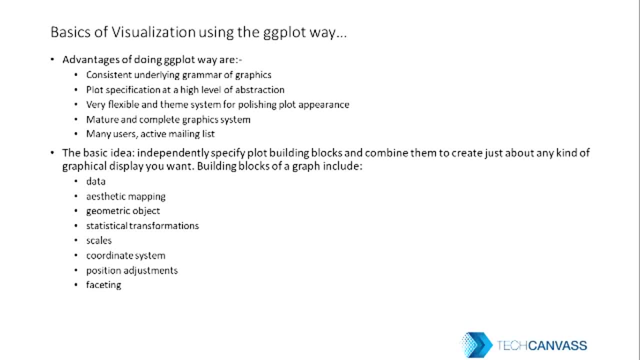 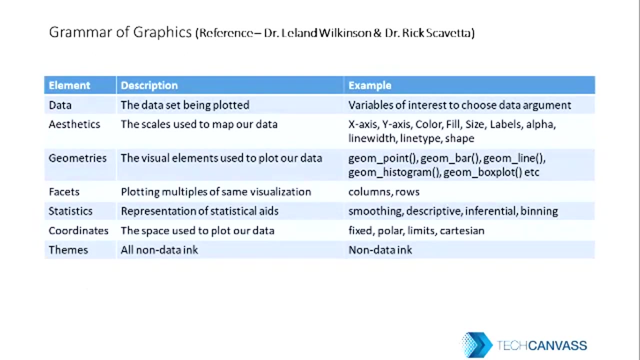 and I'm sure you will find the essence of ggplot2 like others. So let's move on to what is Grammar of Graphics Now. Grammar of Graphics was first described by Dr Leland Wilkinson. There is a book written by Dr Leland Wilkinson. 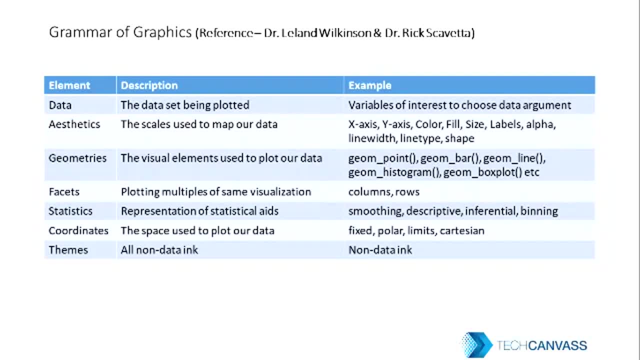 where he talked about the Grammar of Graphics system. It's available on the internet. I don't know if there is a free version available, but Dr Leland Wilkinson was the first person to talk about the Grammar of Graphics based on this concept. 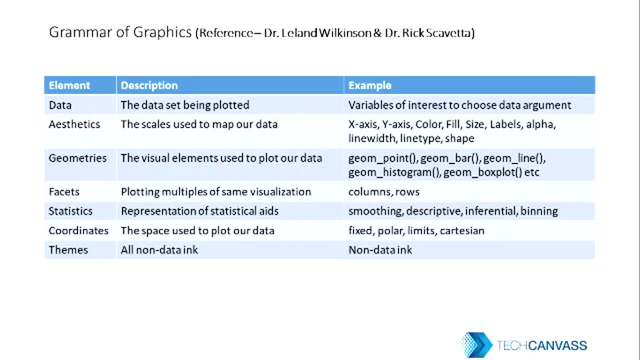 Grammar of Graphics, Hadley, Wickham, built this package, However, the Although Dr Leland Wilkinson invented it, but it was rather spread across the entire universe by Dr Rick Sceveta. Rick Sceveta is a researcher. 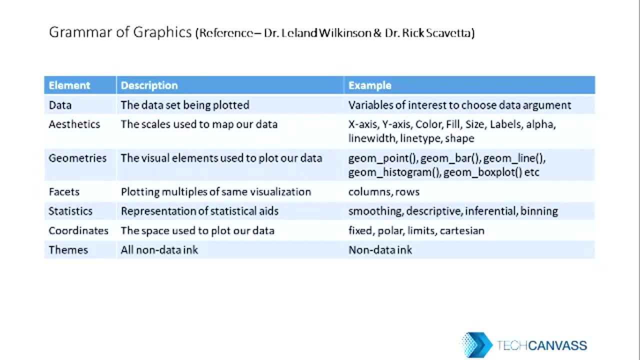 a very, you know, well-known person who has been teaching about gg block 2 functions on several platforms. his book is available on the internet. there are a lot of free materials available by dr rick stevetta and he also is a part of leading training material. you know, leading training portal. 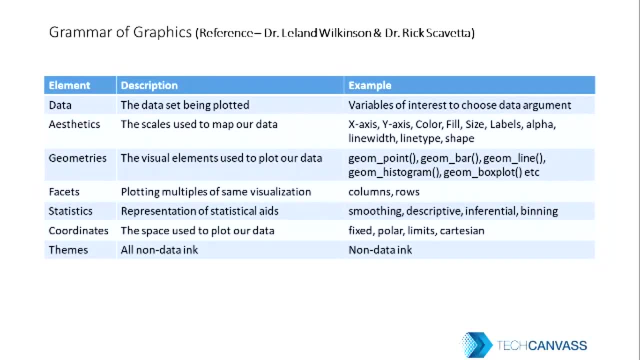 so you can do follow the works of dr rick stevetta as well as hadley wickham and, of course, if you come across the book 11 wilkinson, please do read it, because what i learned myself it's not because of the actual free materials, but i followed these three people who have helped me to learn what i'm. 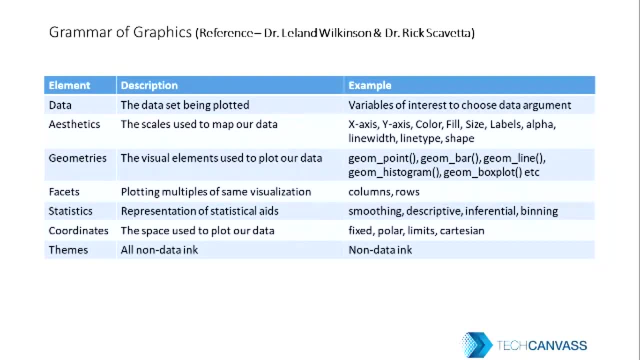 discussing with you today. so these are all the. each row on the table that you see is a layer of the gg block function. first you feed in the data, so the data that needs to be plotted. the data would have variable of interest to choose data argument. next comes the aesthetics part, the scales used to map our data. 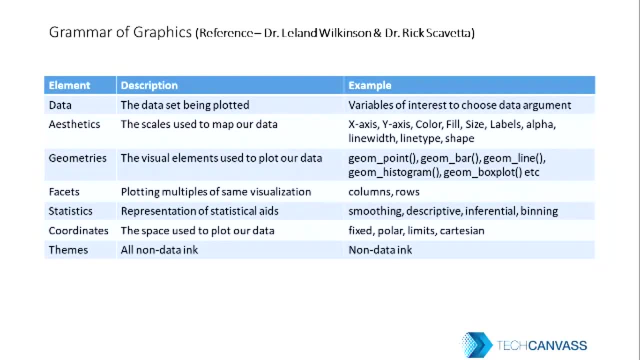 how you use the aesthetics you will see very shortly, right on the next slide. so aesthetics is nothing but x-axis and the y-axis. how you define the axis, which variable goes into which axis, how you define the color, how you define the diameter of the points, the fill size, the labels. 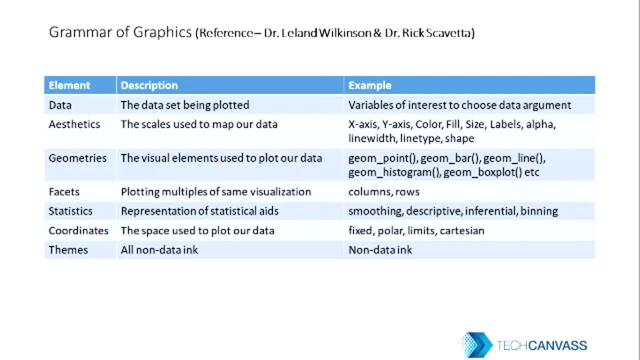 alpha, line width. all of this we will talk about very shortly. what is alpha, what is line width, what is line type? if you are completely new to this, so don't take a back step. i'm sure you have done it somewhere, somehow in a different platform, but maybe not in the same platform, even if you have done it on the. 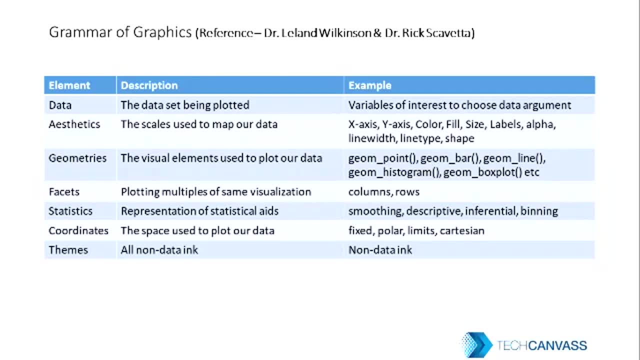 same platform. it would be a good idea to revive with revise ourselves. so what is geometry? the visual elements used to plot our data? it is nothing but all these functions we can use along with the base data and aesthetics layer to get what we want. these are all additional. 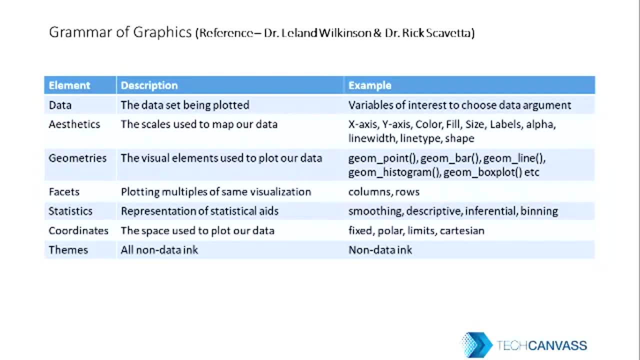 functions that has been used to plot our data and we can use them to plot our data and we can use them, highlighted in geometries, to draw exactly the thing that you want. so point goes for a scatter plot, bar goes for a bar, plot line goes for a line plot. histogram goes for a histogram box plot goes. 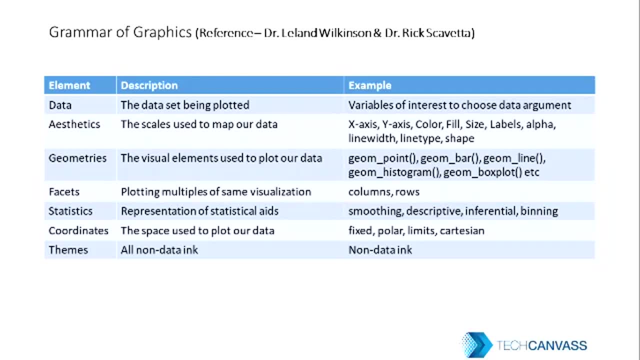 for a box plot, and there are many other things. these are the most common plots that we use in a common day-to-day function, but of course there are different things as well. you can use them based on your need and purpose. so geom is nothing but the geometry. it's a short form of geometry, it's you know this. 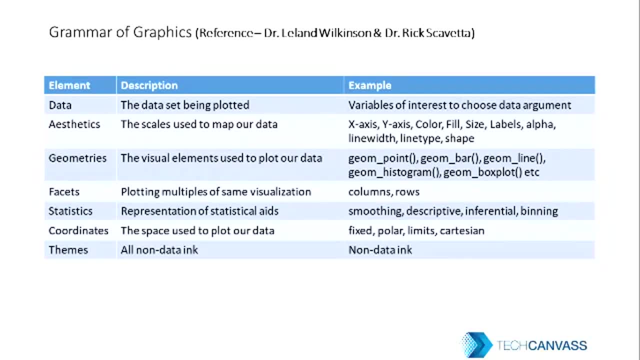 but each function allows you to impose that specific type of chart onto the data and the aesthetics part that you put across. okay, so data, then it sits the aesthetics, on top sits the geometry, then on top of the geometry you have the facet layer. facet layer, you may or may not use every. 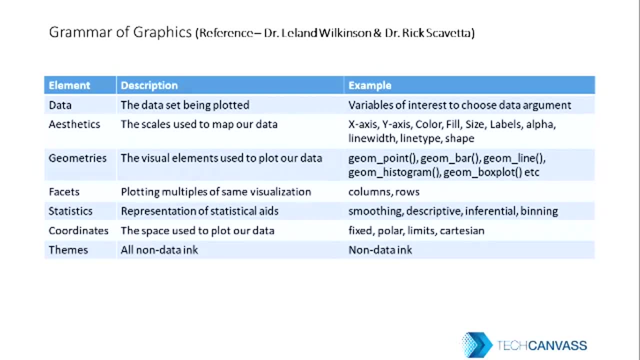 time, depending on the necessity face. it is a little bit more complicated, but you can use it as an example. so by doing this, you can use this to draw a new grid system. you can use it to draw a new grid system. you can use it to draw a new grid system. you can use it to draw a new grid system. 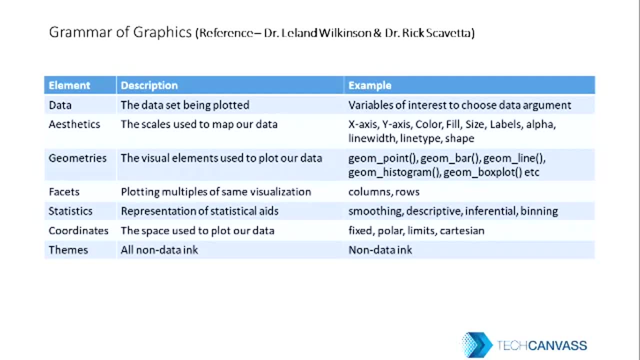 by row or by column so that it looks more visible, more interpretable. okay, you have the statistics function like smoothing descriptive. you can draw a smooth line, the best fit regression line, which we will talk about today. we have read that in books, maybe somewhere, but we can easily draw. 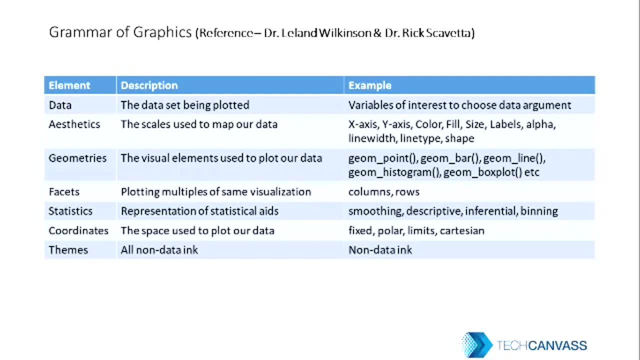 a best fit regression line, depending on the points or the data points that we have in our data set. next comes the coordinate system. it's not too much that we use in our day-to-day function, but if there is a need to flip the coordinates, like you, 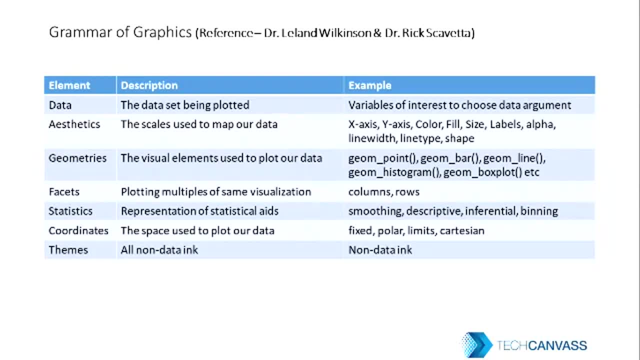 know, normally it is fixed by default, but if we want to limit the coordinates, if we want to flip the coordinates, we can definitely use that. next comes the themes. themes is nothing, but anything that is not related to the data is theme. anything that is not related to the data, okay. that's why I say all non. 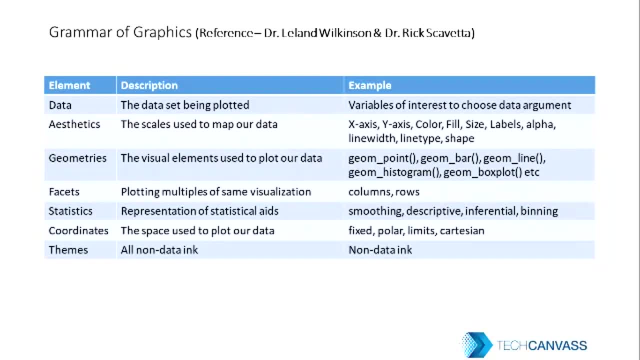 data in anything that is not related to the data, is what is not related to the data: the color of the line, the color of the background, the appearance of the background, the appearance of the. you know the grid where the plotting is happening. you know the font, the header of the label, of the axes, of the exact data. 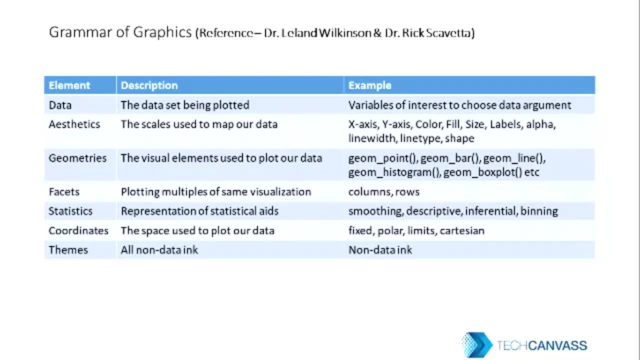 points that gets plot on the x-axis and y-axis. all those that's not related to the data. all the aesthetics part, all the things that we used to modify with a sketch pen in our school days. back in our school days we used to make the things bold, italics, then different font. everything that is not related to the. 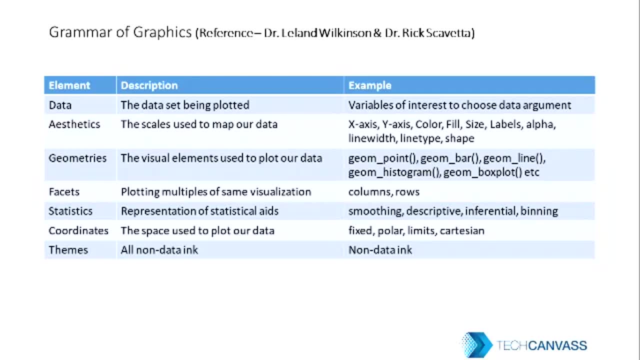 data belongs to key. okay, now aesthetics. please do keep in mind this is one of the most important stuff that we will use in ggplot: x-axis, y-axis. this function needs to know. other than that, it's very difficult for this function. you don't really need to mention what is x-axis, what is y-axis all the time, but 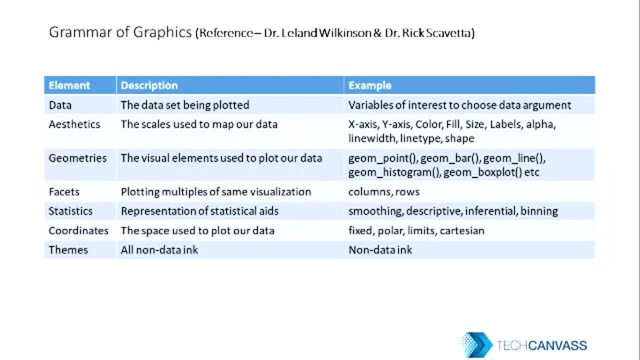 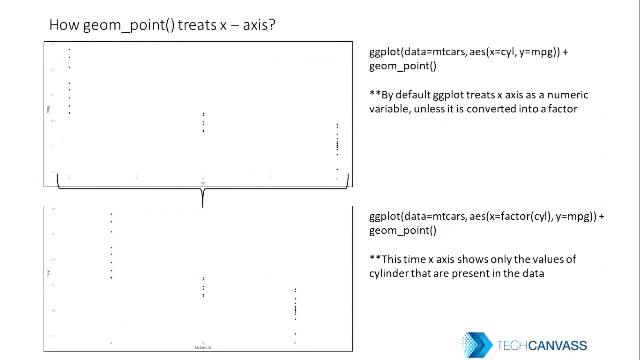 by default x and y. it's comes first and then comes y. if you move the order, it becomes easy to map the data. okay, so quickly move on to the slide. how to point? treats x-axis, so each slide would have the code corresponding with which have been used to plot the data. the data set is available the moment you. 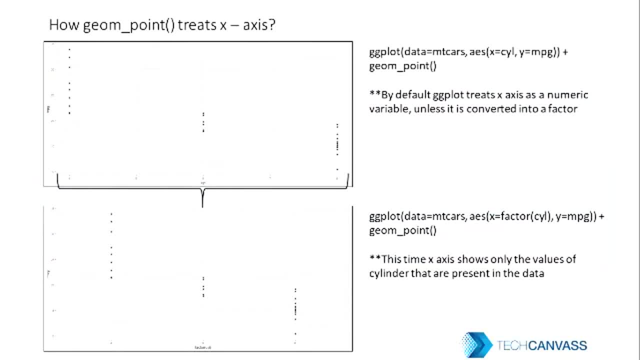 download the package. this is a free data set. I'm not using it, I'm not modifying it. I'm not using it. I'm not modifying it. I'm not modifying it. I'm not modifying anything on this data set. the moment you download the packet, the data set. 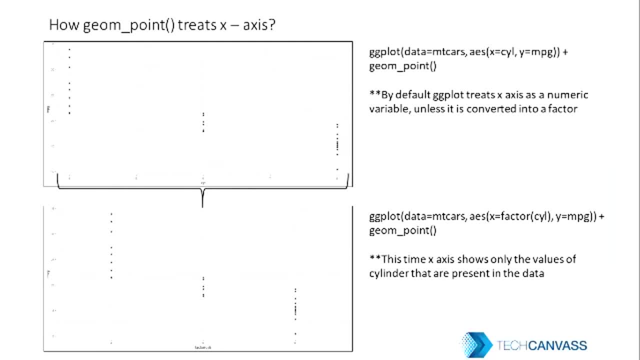 also is available. you can try it on your system and see how it looks on your system. but to understand the concept, look at how the first chart is being made: ggplot. that's the data in the aesthetics part. the data is the empty parts data center using the aesthetics, which is a short form of AES. that begins. 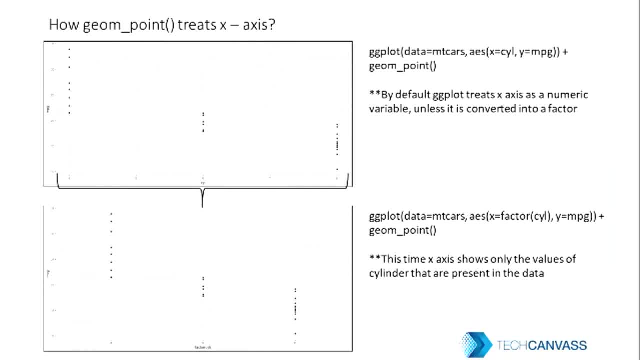 with the first bracket. within the first bracket, we always need to mention X and followed by the Y. okay, so always remember: the X comes first, the Y comes up next second. no matter what ggplot functions we are using, no matter what geometries we are using, we can also use the aesthetics inside specific geom. 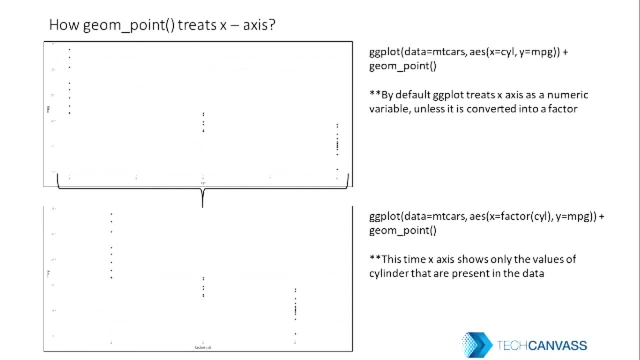 functions. however, just to understand the initial part, this is how the function gets built. the aesthetics comes next to the data and once the aesthetics and data are defined, we wrap data and aesthetics inside the ggplot and then add a plus sign to add the specific scatter plot. so I wanted a scatter plot. 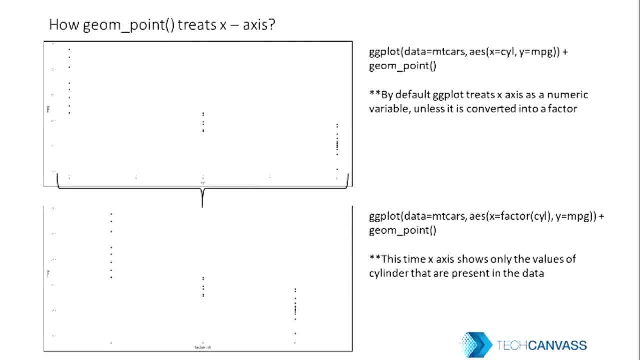 out of this data. I'm adding a geom point function. okay, but by default see that cylinder is a numeric data. okay, cylinder, if you look at the data set structure, cylinder is a numeric data. so that's why you see on the first plot you have five in between four and six. I don't know how big it looks on your vision problem. 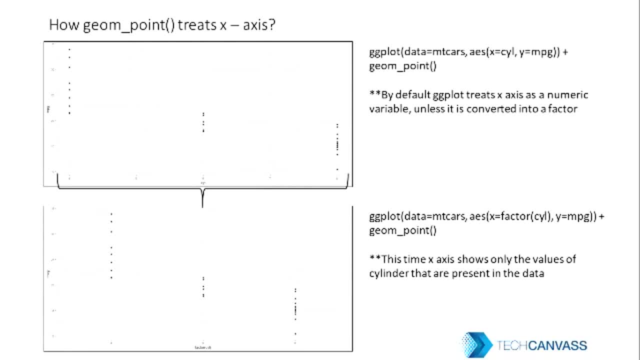 but that's the best I could fit this chance. so for five comes in between four and six, seven comes in between six and eight. so you see, extra data points have been plotted. so that's because ggplot by default treats a numeric scale and on the X, if you put, if you are putting the numeric scale, whichever I have put, 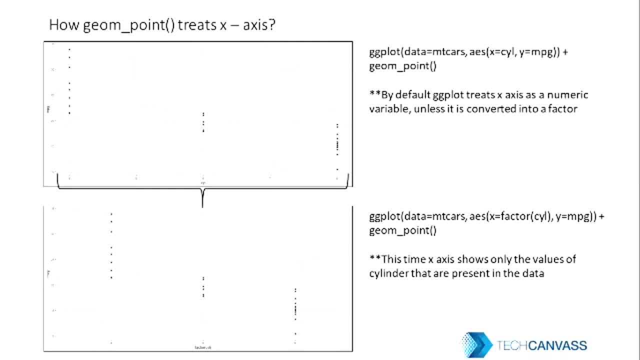 X as cylinder. by default it will plot it in a numeric method, but if you don't want the unwanted numbers, you have to convert it into a factor, which you see on the second graph. I have used a factor function. what exactly the factor function is doing? it is saying that there are only three levels in the data: four, six. 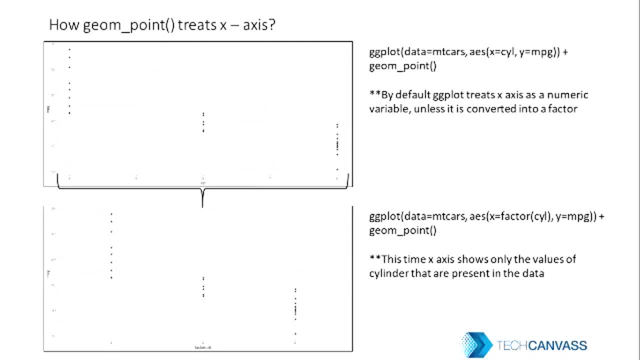 and eight. we don't need any other unnecessary numerical levels like five and seven, so that we only need to see four, six and eight in the chart. we don't want to see the other numbers. so factor converts distinct levels in the data and helps it you to. 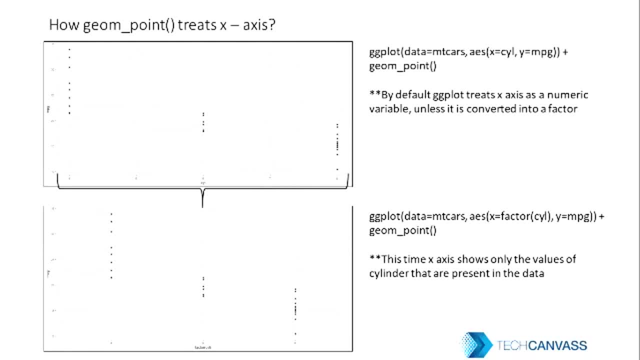 plot in a chart or in a data frame in a table. that's so. the intent of this chart is to see that, by default, ggplot will treat a numerical variable on the x-axis if you, if you are plotting a numerical variable on the x-axis by 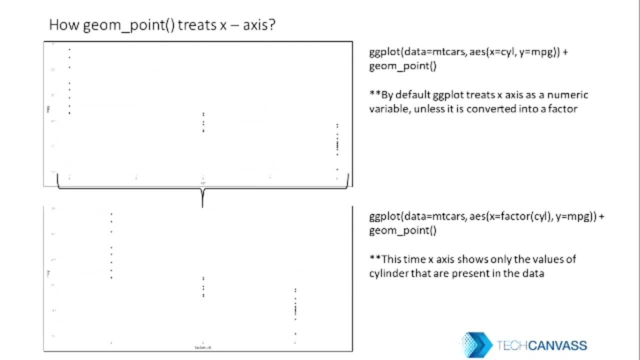 default, all the numbers will get plotted from the minimum to the maximum. but if you don't want the unwanted numbers, please do use a factor function on wrapped around. you know that that particular variable and it could be able to negate that difficulty, okay, so that's why I said this time. x-axis shows only. 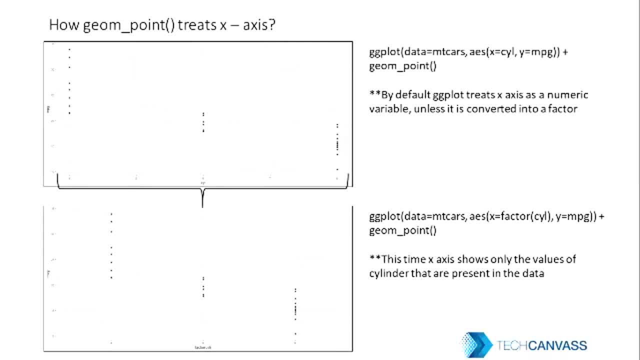 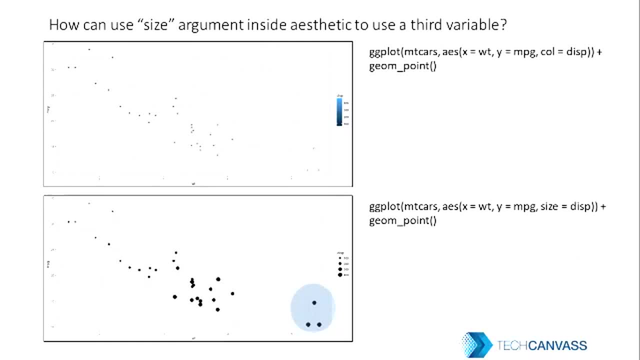 the values of cylinder that are present in the data. next, how can you use size argument inside the aesthetic to a third variable? so see, the x-axis remains the same. okay, I'm using a weight x-axis. on the y-axis we have miles per gallon. okay, both are numeric. this time I didn't necessarily. 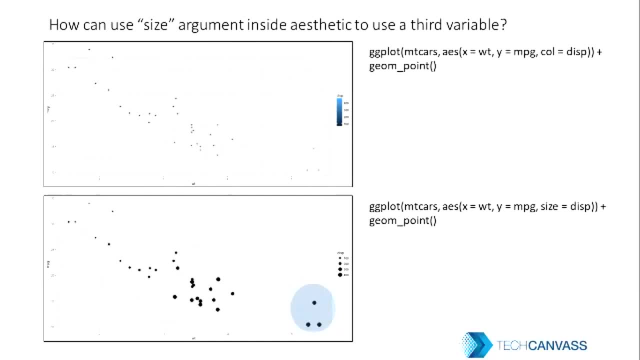 use the factor function because those are the distinct values: two to five. you know the minimum value starts from zero. the maximum ends at, I think, six point five or seven somewhere around that. if you want, you can definitely use it. but weight is a integral scale, so there is no point in using a factor method. it will. 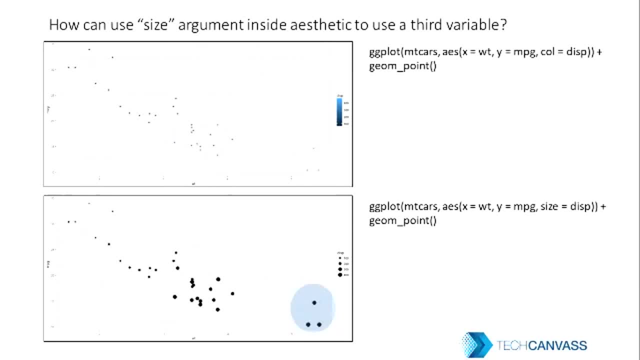 automatically reduce the data. so on the x-axis you have weight, on the y-axis you have miles per gallon. but along with that I wanted to see the relationship of a second very hard variable which is displayed. display is nothing but the display of each car. so what is empty class data set? 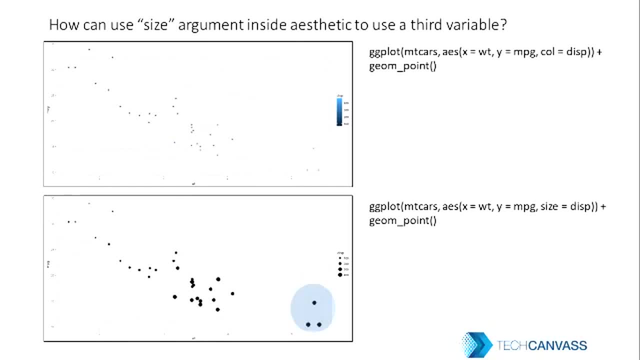 row is a car and each row has different attributes of the car, okay, the engine size, the miles per gallon, the weight of the car, the display size of the car, the different attributes of the car it talks about. so I want to know how weight and miles per gallon relates to each other, but also along with display so you can. 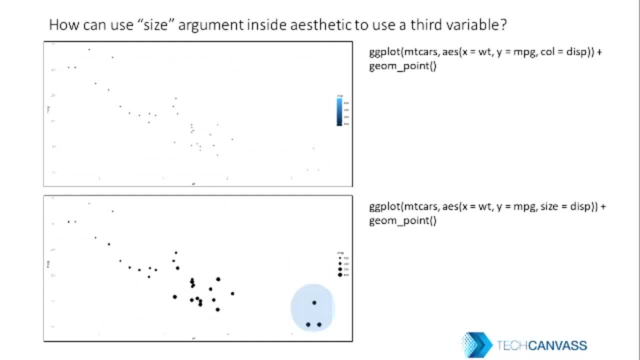 see on the first chart I have small dots appearing based on the color of the display. so since displays a numeric variable, you can see the blue line across that starts from 100 to 400 and the shades keeps changing as the number increases from 100 to 400. but let's say I don't want want it this way, I want to. 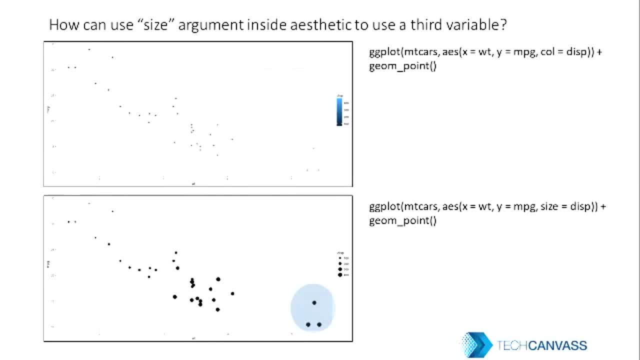 change, the diameter of each point should change along with the levels of display. so that's that's why, instead of color, in the second chart I've used size. okay, so as the value of display increases, the size of the diameter also increases. so from the second chart you can clearly infer that instead of using color, if you use 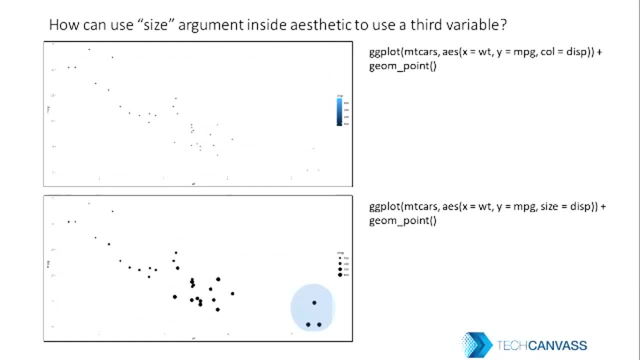 size. so this is the way permutation and combination you need to do what's the best way to interpret the data. ggplot is very useful in interpreting the data rather than giving it a very flashy, you know, cosmetic. so on the x-axis, you see, for the maximum weight, you have the maximum. 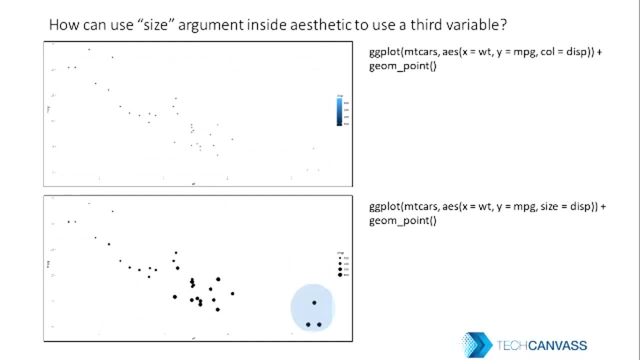 display. so if the weight is also high, display is also high. it directly correlates with the weight and the display, but not necessarily with the minus per gallon. so if you see the highlighted areas, those areas have maximum weight and maximum display okay, whereas if you move to the exactly 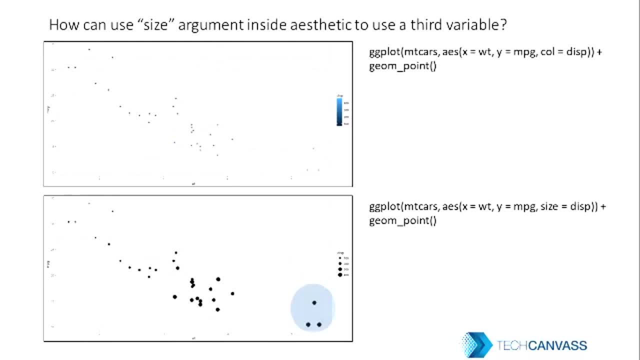 diagonally opposite thing: the weight is minimum, the display is also minimum, whereas the miles per gallon is very high. so there is an inverse, proportional method of miles per gallon to display that. that's a very, you know, high level overview, but definitely being actually coefficients of correlation. talked about it once you. 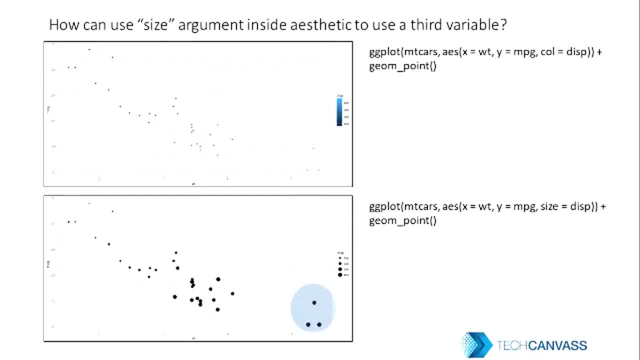 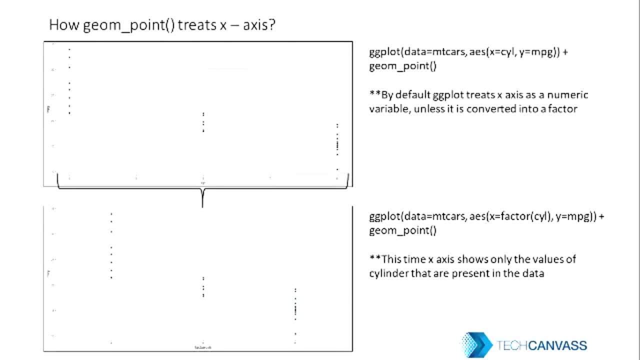 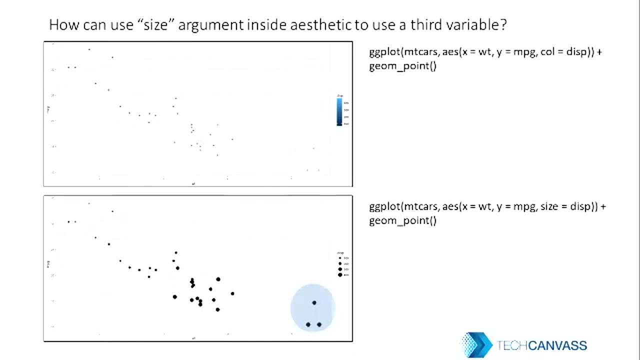 try to find it out. okay, so this is how you can play around the size and color variable. previous slide talked about how you can use the basic functions, but the next slide talks about how you can also use different methods of estimation. so, color argument, size argument, these are all part of aesthetics which you can. 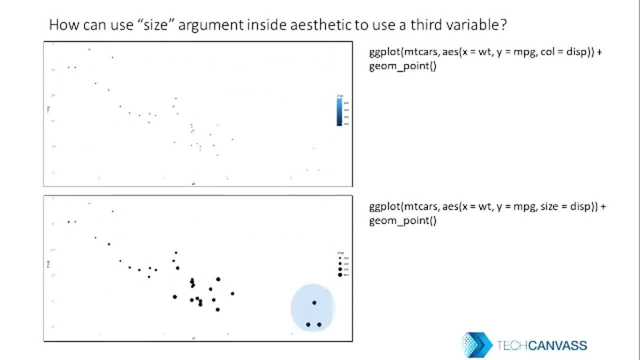 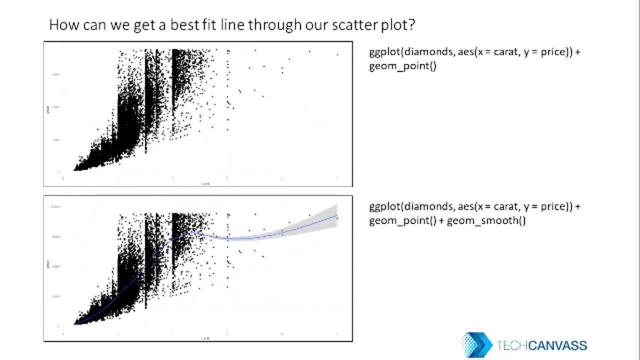 use inside the aesthetic function. okay, next, how we can use a best fit regression line. you see that I am using a different data set. I again use the x-axis, the y-axis, but along with, to your point, I have also used to choose smooth function. it is nothing, but it is a method you can explicitly mention linear. 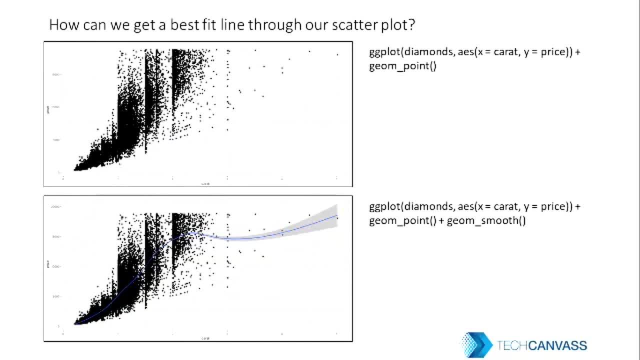 method, or you can explicitly mention maximum likelihood method, LOVSS. so there are different methods of plotting the best line but the by default is LM, which is a linear method. if we use a best fit regression line across all those scatter plots, scatter points, that you okay. 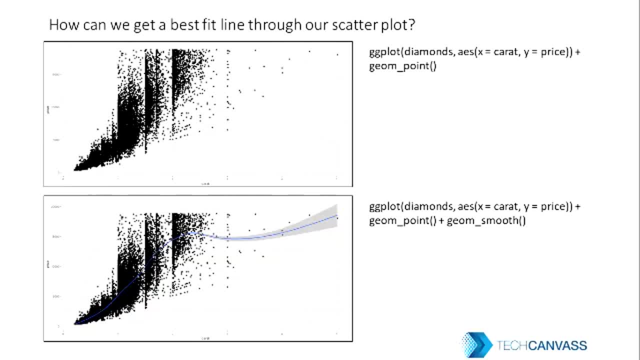 so you know, based on, depending on your study, if you have a training data set or testing data set, you can always use a scatter plot function or a smooth function to understand where exactly the best fit regression line runs or passes through. okay now, although it looks very simple here to use the geom smooth. 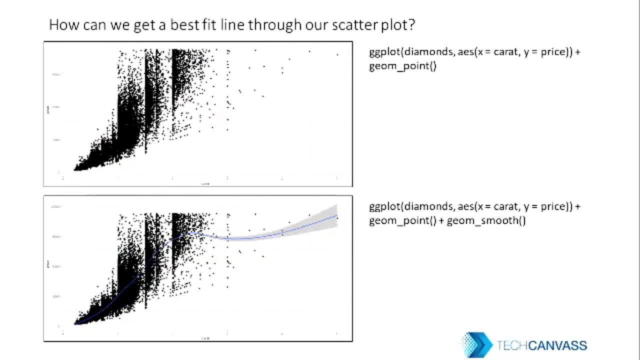 function just by using a plus sign and geom underscore: smooth function. it's very easy that we have got the best fit line. but it is very easy that we have got the best fit line. but it is very easy to do that if you want to replicate the same thing in any other function in 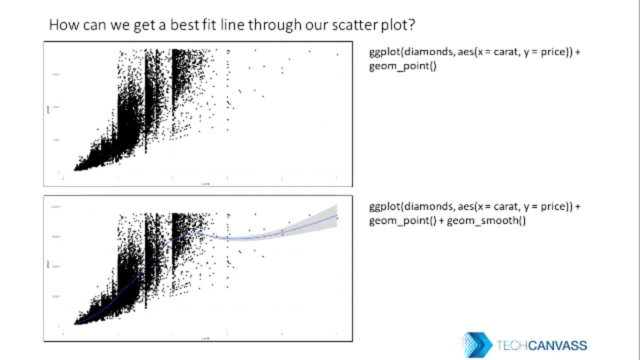 through the basic plot functions. it takes lines and lines of code, lines and lines of, you know, iterations. okay, so this is a very handy tool that we have. so initially it may look that how can such a single function is giving us such a beautiful best fit regression line? but 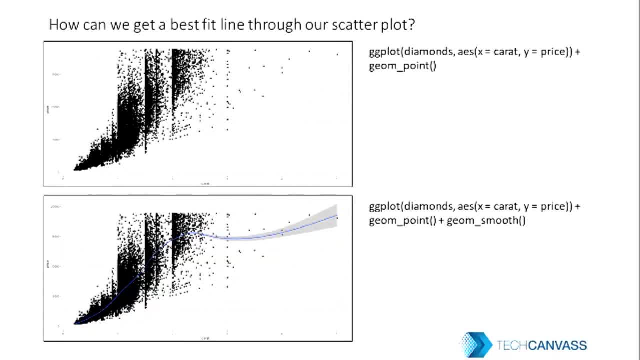 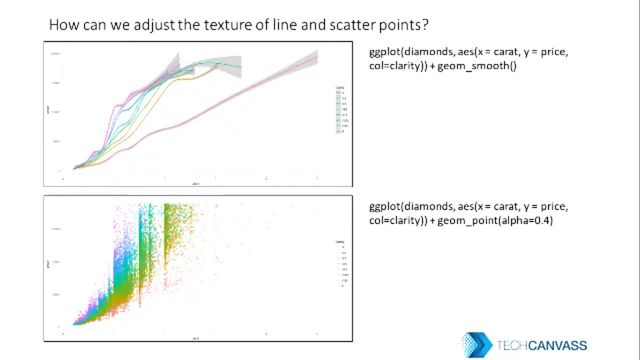 plotting the same thing in these are. it's very, very difficult. I'm not discouraging anyone. if we they want to block the piece are, but I'm just sharing my experience. this is how we can texture the color of the line as well, so you have different groups of clarity. on the x-axis you have the carrot of the 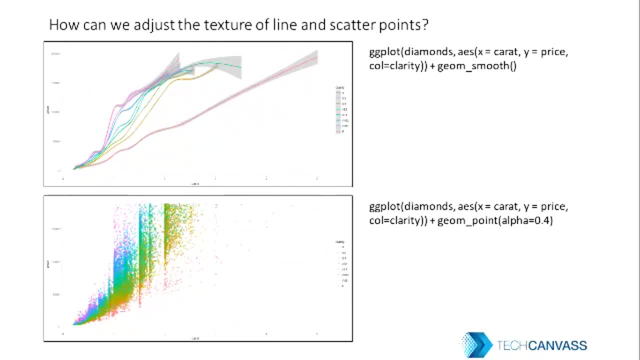 diamond. on the y-axis you have the price of the diamond, but each line also talks about the clarity. so you can see that the line that runs, the very long line that runs from 0 to diagonal all the way, I think that's s1. so any clarity that's been categorized. 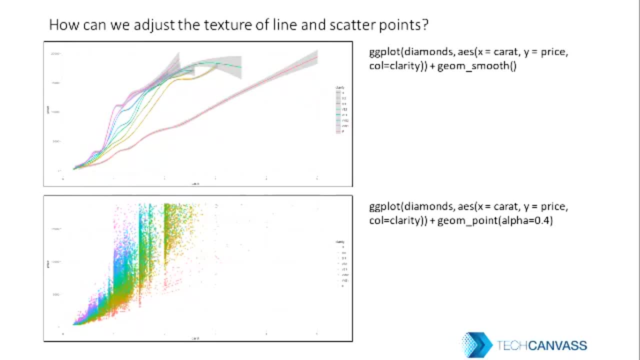 with s1, but that clarity. we have all sorts of carrots ranging from low to high price, but if you look at the clarity, which is if that ends with a carrot of 2.5, and their price is ranges from 0 to around 20,000. okay, so this, these are the various different. 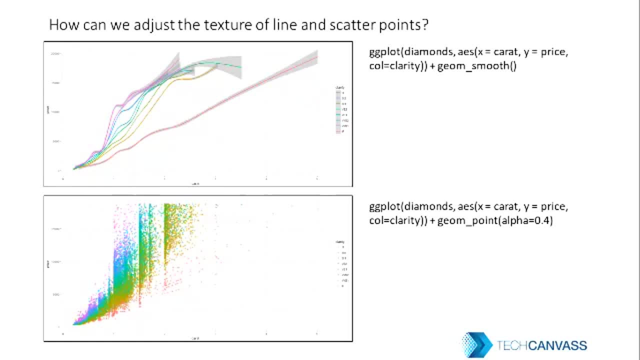 ways of identifying the structure of your data, the content of your data, the characteristics of your data. now, GM smooth function, it will draw a best fit line. but your point, what does the team alpha does in the GM point function? alpha is nothing, but it ranges from 0 to 1: 1 being absolutely dark, okay, 0 being 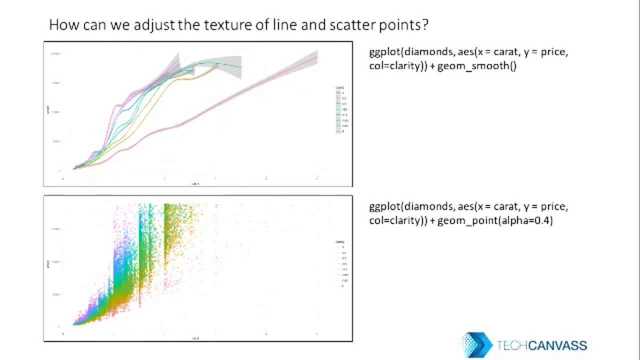 transparent. okay, it's the range of transparent and opaque that you can plot in the chart. so if you see 0.4, you can see the love, the texture of these colors. that scatter plots have become slightly blurry. you can use it to understand if they are lying on top of each other. 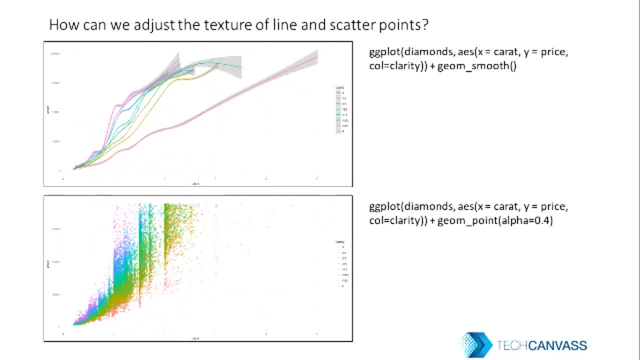 so you can see the green color sits on top of the blue. so it's not necessarily. you know. you can infer that there is no data point. so obviously there is data point. but you can vary the alpha figure to identify whether there is actual data inside it or not. so alpha is nothing but the range of 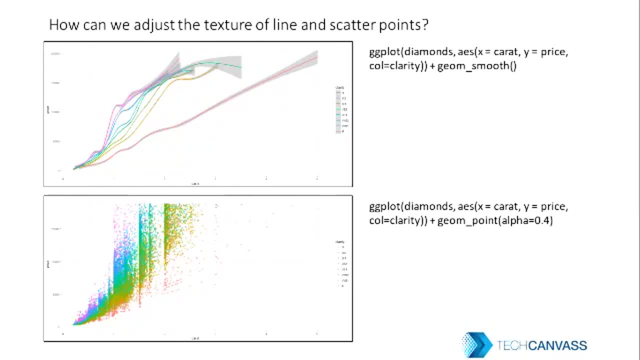 transparency to go big. you can vary the you know shade color. so you can see the green color sits on top of the blue. so it's not color, not exactly the color, but the shade of the color through alpha. okay, next some more examples of GM point and GM smooth combination. so GM smooth. 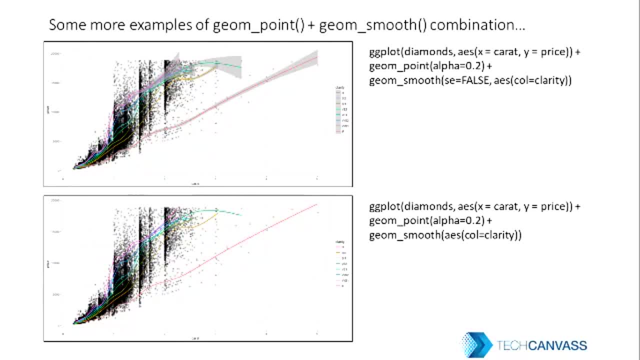 always runs with GM point. please keep this in mind. your point is nothing, but you know, modification of clad scatter plot. for using scatter plot you use GM point. alpha is equal to 0.2. that means I want a very, you know, transfering very opaque stuff. one means: 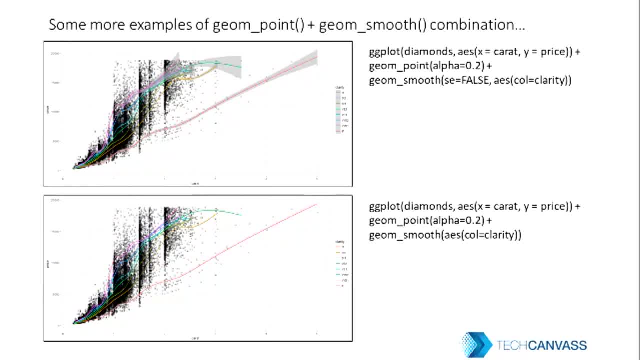 keep on making it bloody. that's it. so this is how you can see. so the next example: you can see that I'm using Jim smooth and within June smooth you have a yes color is equal to clarity. so what, what basically does is, on the first aesthetic function I'm using, what is the x-axis in the? 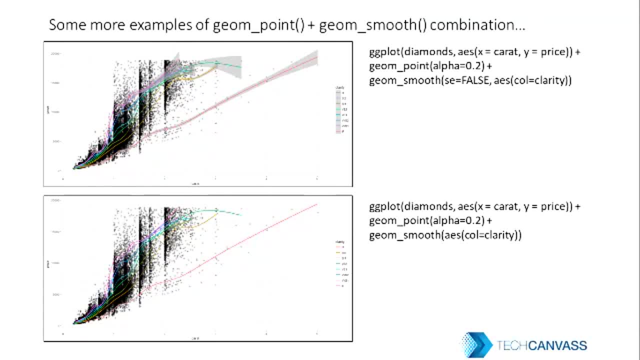 the y-axis on the second geo point, I'm using the texture of the point, but in the June smooth I am deliberately mentioning, the color is equal to clarity, so that the color of the best bit line sits on top of the actual scatter blocks. which is which, which, which? which didn't happen in the first plot, okay, which? 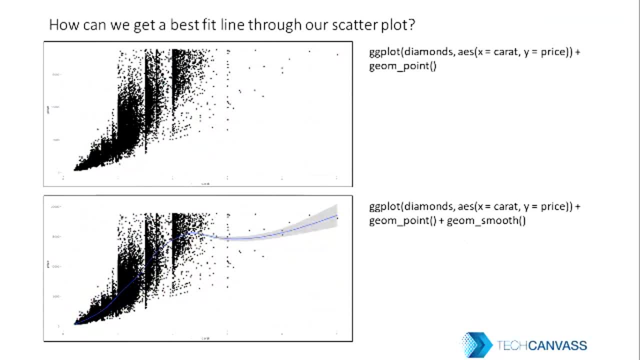 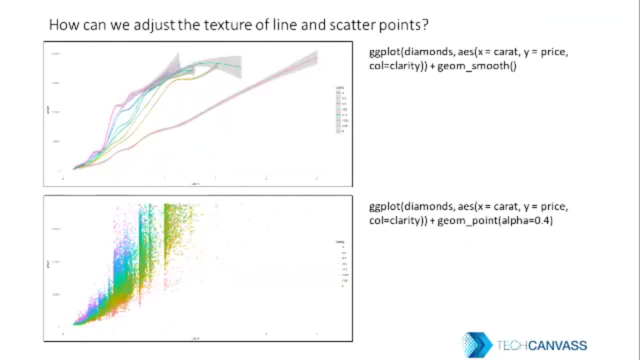 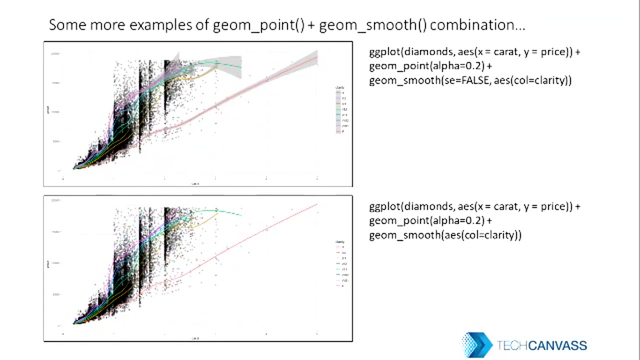 didn't happen here. okay, the smooth did lie on top of the gym point, but there are areas which becomes indistinct if you don't mention the AES function inside the gym smooth. so this method is a bit more clarified method. the lines that the cut lines of the color would sit on top of the actual scatter plots. 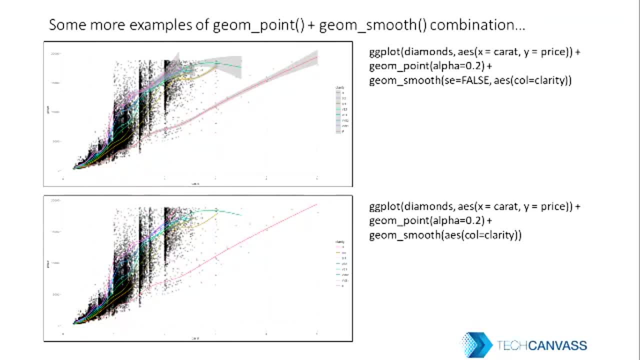 so that it's just like a graph paper that you draw in a union of school days. you first put the dots on your graph paper and then you draw the best fit regression line on which which runs on top of those points, so that it becomes very clearly evident where exactly that line is originating from and what's the. 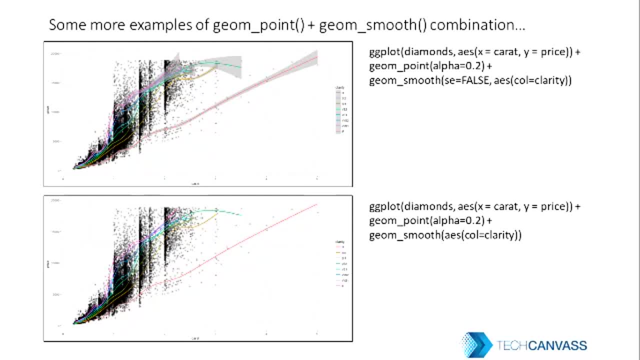 direction of that line. so you can also use AES function in inside other geometrical functions. but this particular example I wanted to give, that if you have a graph paper and you draw the best fit regression line on top of you, if you'll have a set of points, you can draw a line on top of those points. 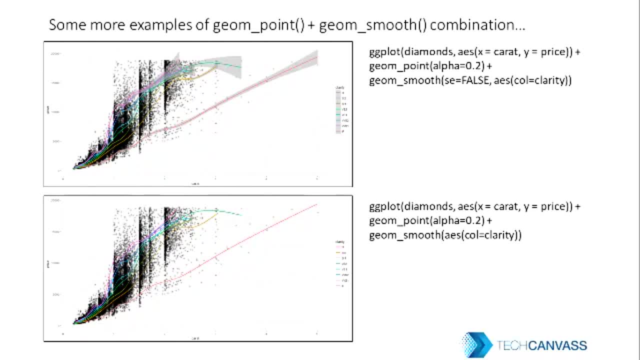 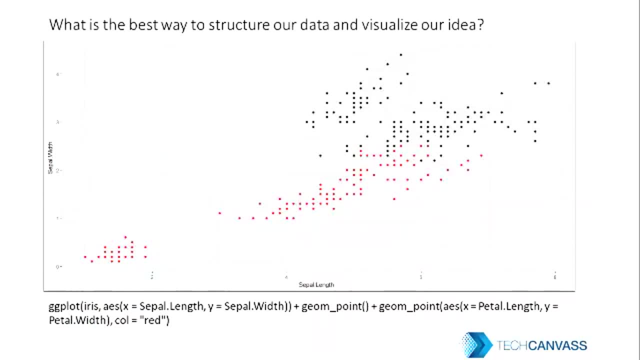 function. if you have a set points, you can draw a line on top of those points as well by using AS function. ok, the next comes. so this is a very practical example that code lies below the the chart actually. so this is an iris data. this is a very practical example that code lies below the the chart actually. 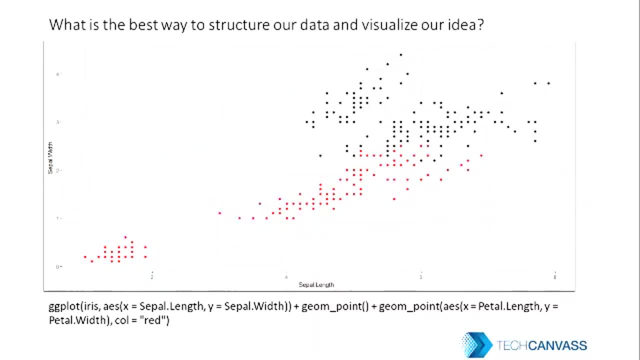 set. this is also a free data set. if you look at the iris data set from your, consequently will find that it has four variables. it here is no oneそれ four variables and you can't need to rewrite an extra one because now you are found that you were. so if you don't know that data set from a node in your one. 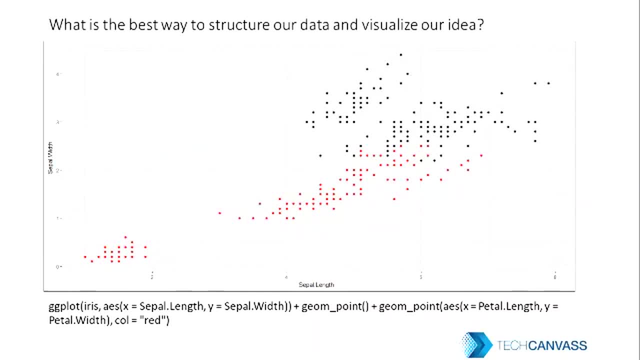 concept. but if you yaw your molto part, you will find that it is going to automatically Butterfly grid. you will find that it has the mosthst thì I will. it comes up your. it has got two kinds of length, which is- somebody has a question? the one did: somebody has a question. 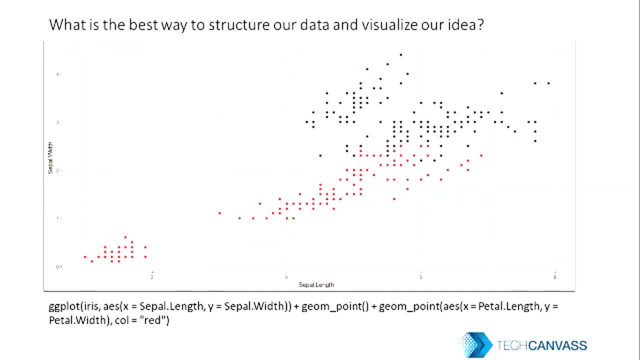 i don't know, shall i move on? or somebody went unmute, so okay. so we have the uh iris data set. you will notice that you have two different kinds of length and two different kinds of width. okay, now it's very difficult on a two-dimensional architecture to 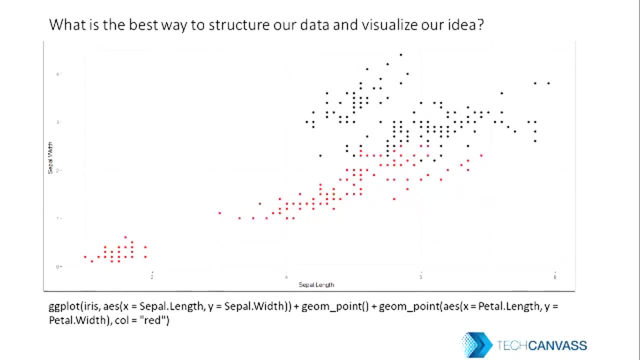 figure out how you will plot or how you will identify the length and the width of both the beetles and the sepals. okay, so if you do, if you use the basic method of ggplot, you will see that the iris data set goes in the data section. in the aes section i'm using the 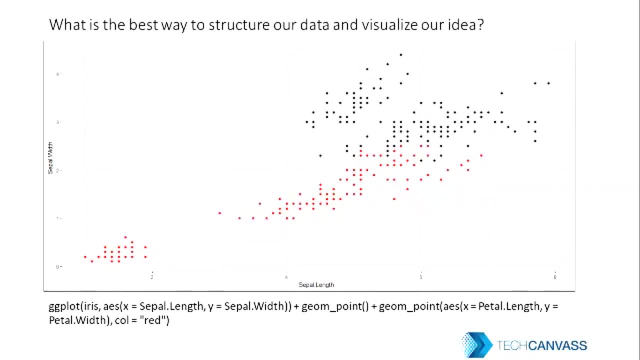 sepal length and the sepal width. that's why the axis get labeled as sepal length and the sepal width on top of it. i'm using a gm point function which is a scatter plot the relationship between the length and the width of the sepals. 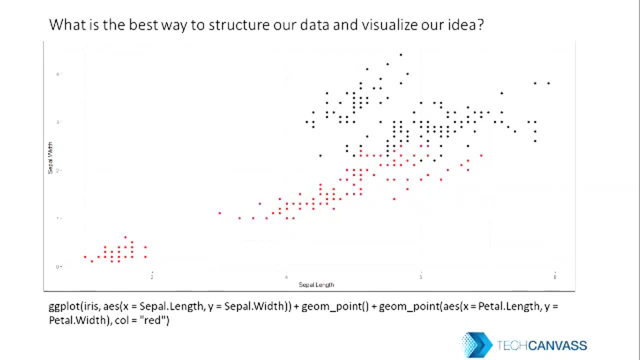 what next i'm doing is i'm again using a point function to identify, or rather to explicitly mention, what is peter length and what is the width, and put that, or rather color those dots as red. so you see that, whatever red dots, those are the characteristics of the beetles. 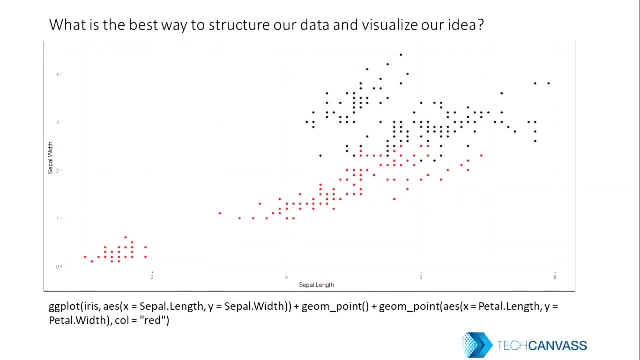 but the black dots. those are the characteristics of the sepals, but you don't have any method to put the label as sepal length. you can obviously explicitly mention that the x-axis is sepal length and peter length. you can also mention sepal width and. 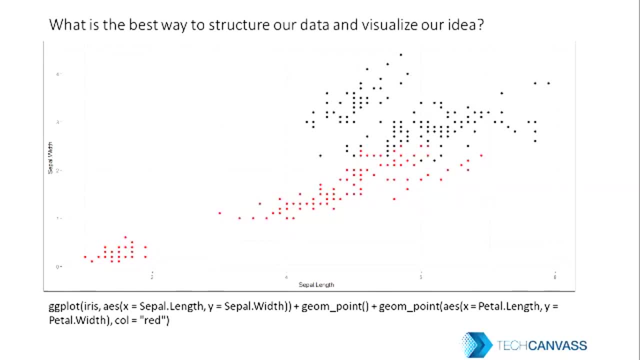 peter width, but you cannot put a legend here, because it's very difficult that you are plotting all the four variables and then trying to identify the relation. so this is a very good example of how to structure your data. okay, how am i structuring the data to identify what exactly i want? so, what exactly i want? 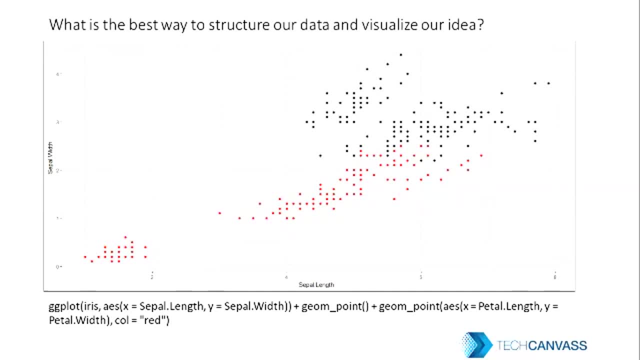 from this example. this is not the chart that i want to know. what i want to know is how the length and width varies across all the species of flowers. that goes inside the iris data set. i want to know the sepal. i want length. i want to know the peter length. 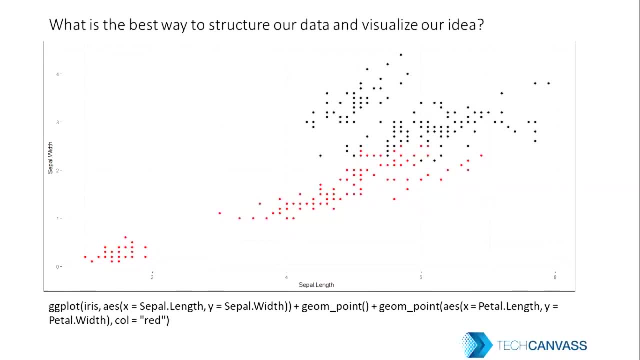 as well as the same for width as well, and i'm also. this method doesn't allow me to bifurcate across the species, but only bifurcating across the variables, that is, that's there in the data. so this is a very good method of using. 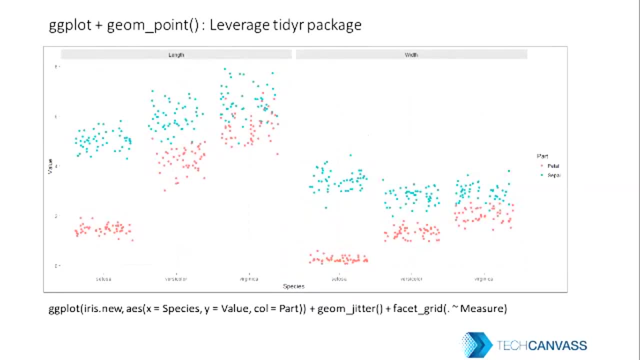 the tidy art package. the actual code to create that data set has been put in the notes section. this is also readily available on the internet as well. but look at what's the intent of the chart, the first chart this is faceting. okay, on one chart, i am. 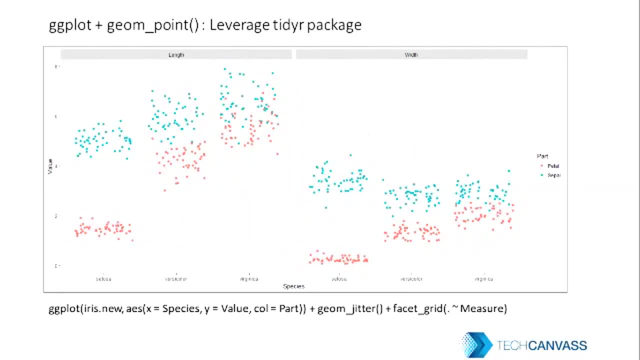 bifurcating two. the first chart talks about the length, the second about the width. on each x-axis you have the species setosa versicolor and virginica. on the y-axis you have the value. so you can clearly distinguish that the red color belongs to the beetle, the blue color belongs to the sepal. 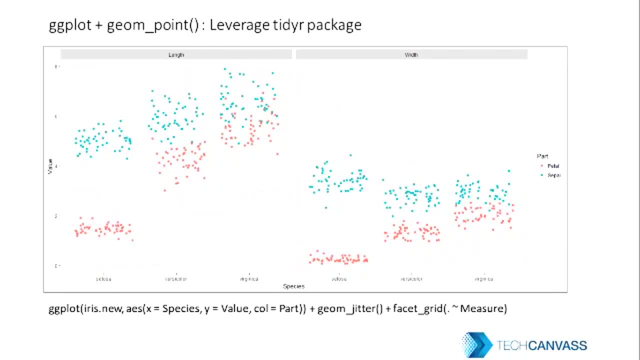 whereas length is considered the length of setosa. the petal length for setosa is lower than the sepal length, and that holds true for versicolor and virginica, whereas the width- the petal width- of setosa is lesser than the sepal width of. 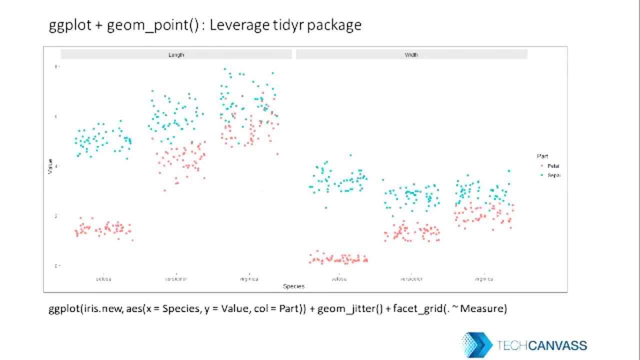 petosa, and that also holds true for all the three species. but the only breaking difference is the length, both the sepal length and the petal length, the sepal width and the petal, i would say sepal and uh, you know the the length of sepals and petals are. 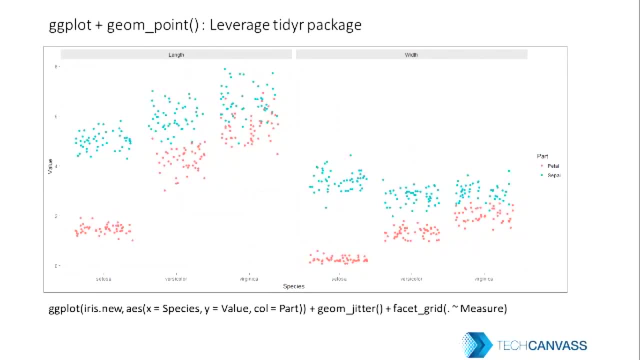 distinctively higher for virginica, but for when it comes to width- the sepal width and the petal width- they are almost similar to versicolor. okay, so, as you see that you can clearly distinguish, you can derive more characteristics of your scatter plot. you can do more of your data analysis by simply using. 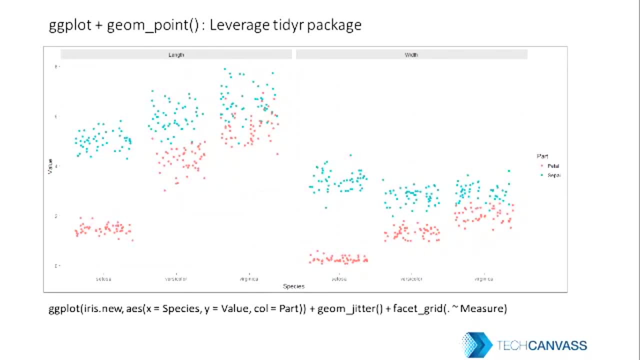 the tidier packet, how i'm using the idr packets. that's actually mentioned in the notes that you can see in the notes section of this slide. but the code that sits on top, just below the chart, is the actual code that is required to build a chart. but behind this chart there also goes a 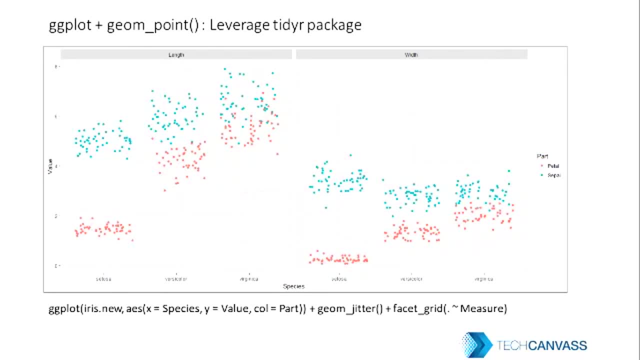 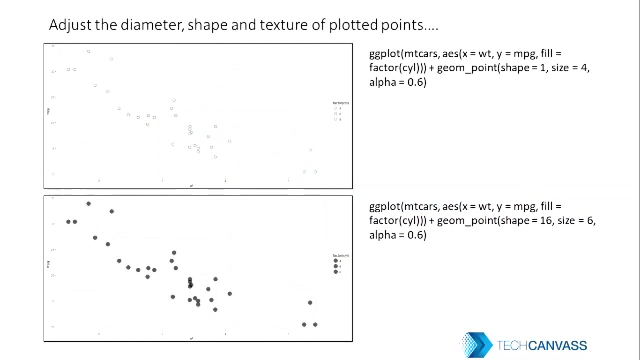 data set, which is iris new. okay, how to create the iris new you can know from the slide. okay, so this is one way of identifying scatter plot. next is adjusting the diameter, the shape and the texture you have. you can use the shape, the size, the alpha together to characterize the. 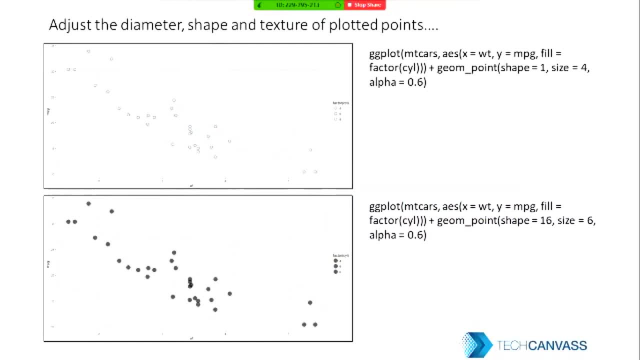 diameter of the plot, the texture of the plots. you know the actual point that gets plotted, mind you, not anything that is non-data is the theme, but anything related to the data is actually needs, you know, actually needs to go inside the geometrical or aesthetic function. so 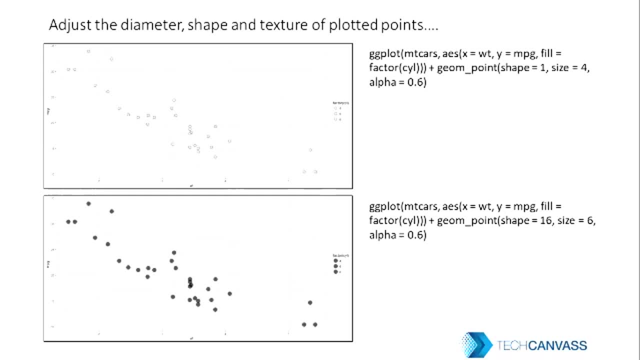 shape is equal to one means the diameter of the point that you see. shape is equal to 16. you can see the diameter of the point has actually increased. size is equal to 4 means the actual size of the points. it is not necessarily the diameter, but 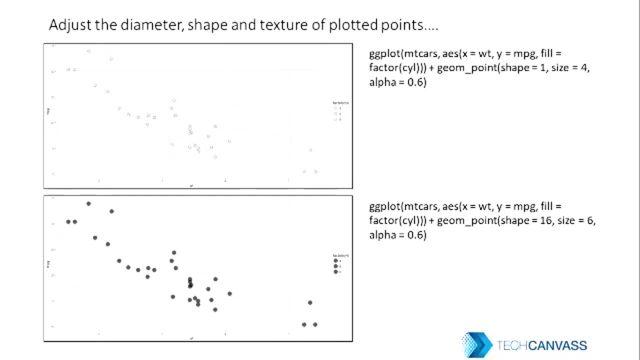 shape would give you a circle, whereas the size would give you the actual diameter. okay, you can keep trying different shapes, but along with the shape and size, you can keep varying them. you, you can create triangle, you can create boxes, you can try all sorts of things. so 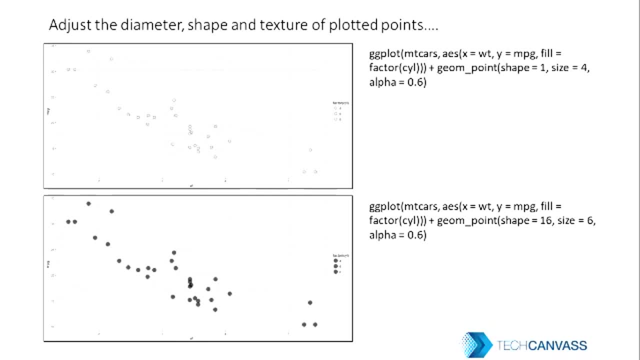 shape and size together give you a different little feel. so shape and size go together. okay. alpha is also, as i talked about, used to derive the texture as well. okay, next slide is adjusting the diameter and shape. again a different example of shape and size. along with the alpha, you can keep varying the color. 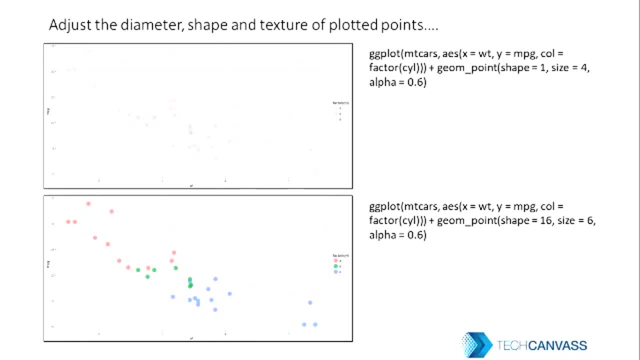 argument to see how it looks. so if you just use shape one and size is equal to four, you have small. you know, a little bit difficult to read the points, but you can also increase the size and the shape. the points become a little more visible, okay, next is: uh, you can manually mention the color. 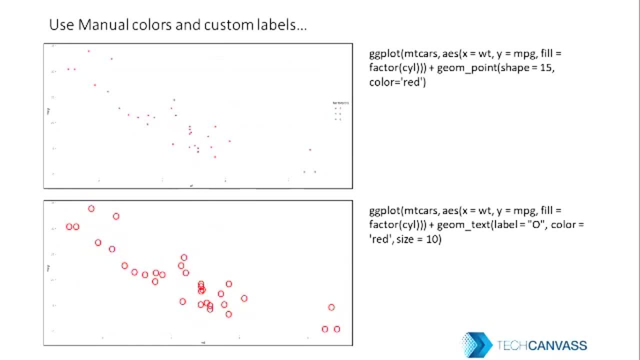 as well. so you can see that i have used level label argument. uh, with an o you can, instead of o, you can put any letter as well: a to z, whatever you want. so the points that you see on the second plot is nothing but the alphabet o. so instead of o, you can type a. 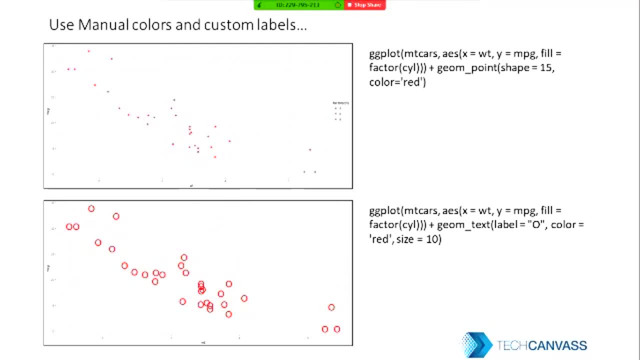 x, y, anything, those, those, those characters will be plotted. you can also mention an explicit color argument inside the geometry functions to change the color. if you don't, if you, if you don't like, uh, the actual default color. so on the first chart you see the shape. 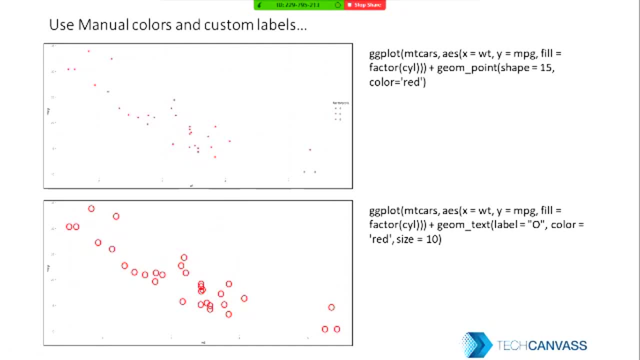 is equal to 15. actually i think has given square points, data points, it becomes very small. but if you really go inside, shape is equal to 15 is a square structure. all the points would look like a square. but if you explicitly mention the label argument inside the geom text, 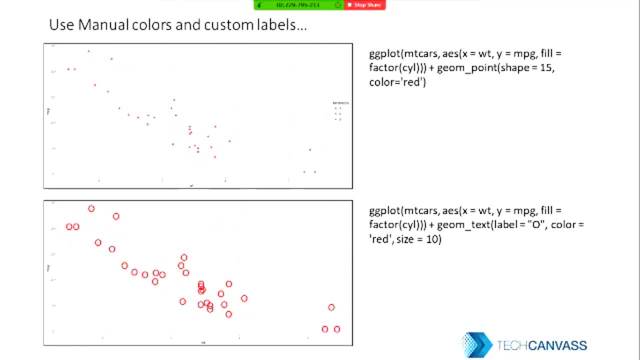 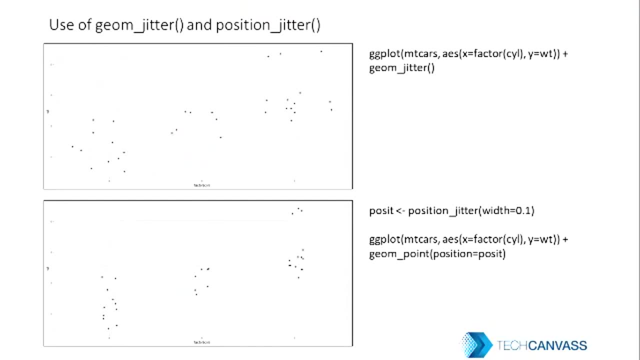 you can plot anything that you want. next is the jittery function and the position jitter function. this is a very important concept when plotting scatter plots. if you see, by default you use geom jitter. the x axis has 4, 6 and 8, but the points are scattered. okay, but you want. 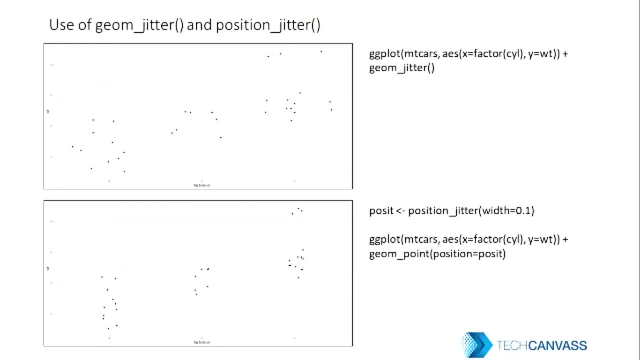 points to be a little bit distributed so you can use a position jitter with this equal to argument position jitter. width is is nothing but the amount of, but reducing the width of the axis that it takes. On the first chart the points are taking a lot of space. 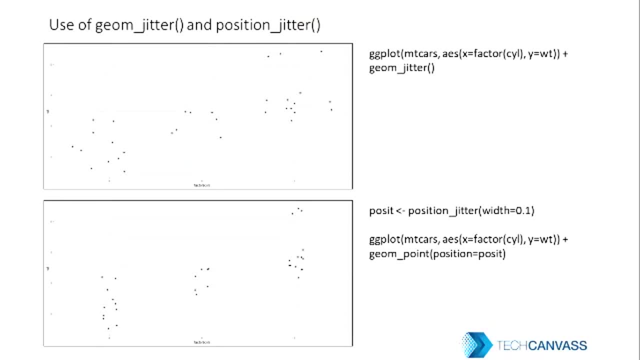 to get plotted, whereas if you use position ditter, the actual geometry of the dimension gets reduced, but the actual data values doesn't change. The relationship doesn't change. the actual data values doesn't change, it's just the structure of the plotting that gets changed. 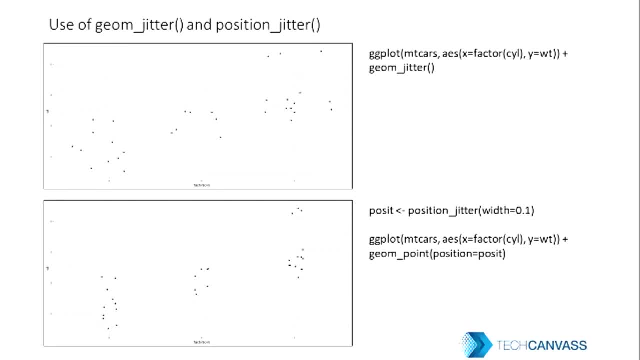 It becomes visibly more attractive. So position ditter is a very useful and common argument that gets used in day-to-day scatter plots. If you have in the second chart you have four, six and eight, it's easily readable. but if you have more than four, five or 10 data points, 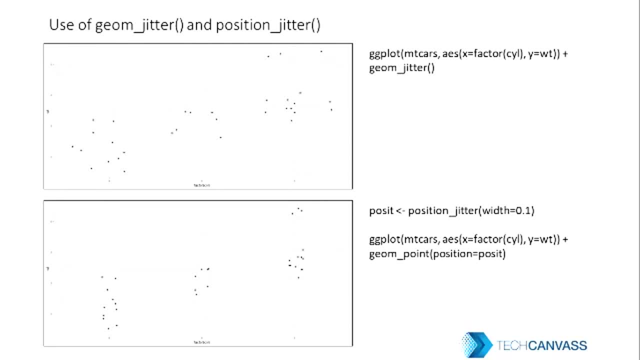 no position. ditter is a good method to use so that one data point doesn't overlap with each other. So the actual code has been given on every slide. You can keep practicing it in your leisure time. Next comes the histogram, one of the easiest way. 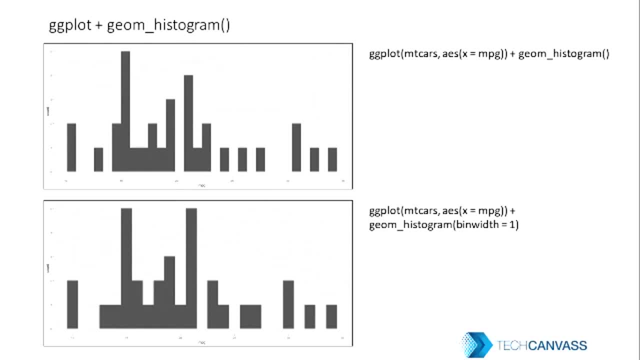 to plot the histogram in R. You just need to mention the histogram and obviously the histogram takes only one axis. so that's why the x-axis comes first. Using miles per gallon- you can use the weight as well- Bin width- bin width is nothing but each bin. 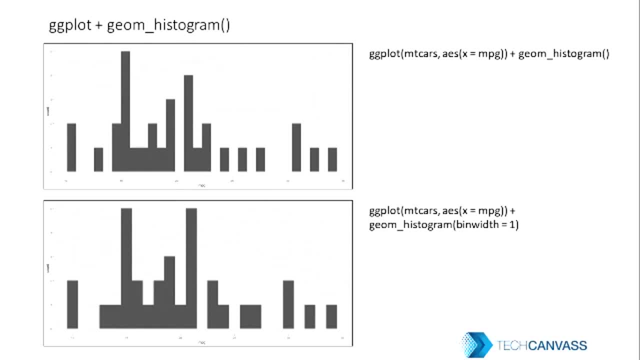 will have a width of one. So that means you see, in the first chart, the x-axis, the bar starts from 10.. However, if you look at the actual data, there are values for miles per gallon which are below 10.. 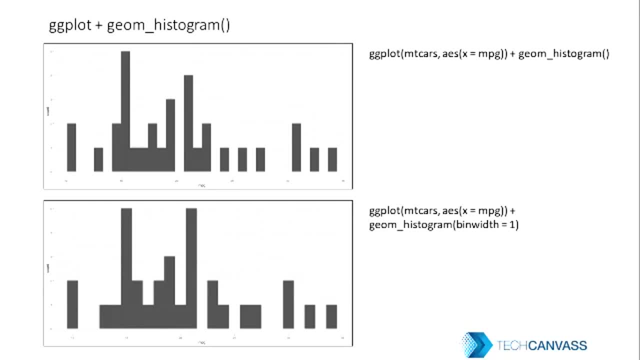 So when I'm saying bin width is equal to one, I'm saying: keep the bin width as one so that it becomes 10 to 11,, 11 to 12,, 12 to 13,, 13 to 14, that way okay. 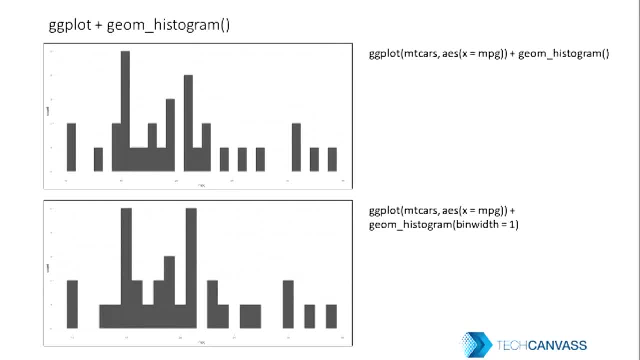 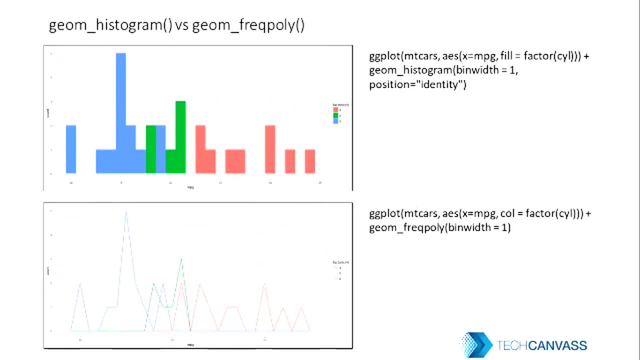 So you can keep playing with the bin width and see how the histogram gets plotted. This is nothing but changing the color of the histogram based on the cylinder variable. So you are actually measuring miles per gallon and the count of the frequencies on the miles per gallon. 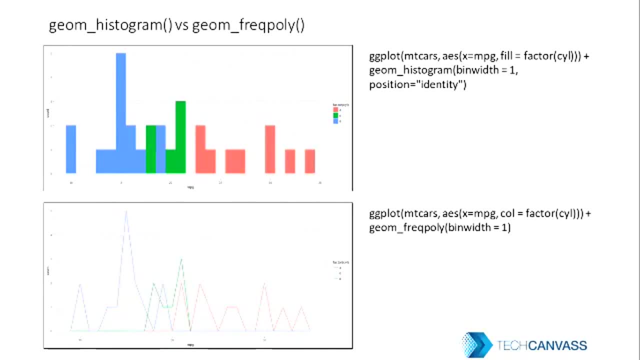 but also you want to plot the cylinder. You want to see how the relationship goes with cylinders. So you can see if the cylinder is four, if it's of size four, then the miles per gallon is very high, whereas if the cylinder is of eight, 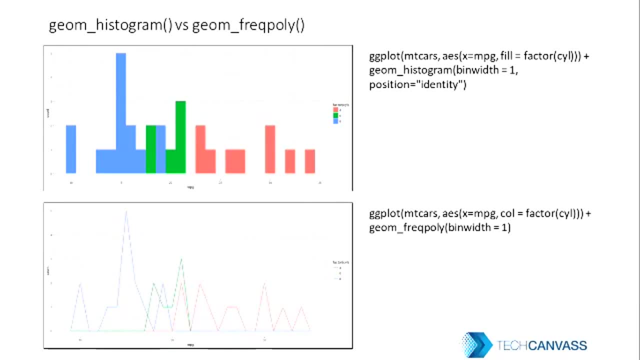 then the miles per gallon ends somewhere around 18, which is obvious, because if the cylinder size is high, then obviously the mileage will be less. If the cylinder size is low, the mileage will be very high. The next plot is a free poly plot. 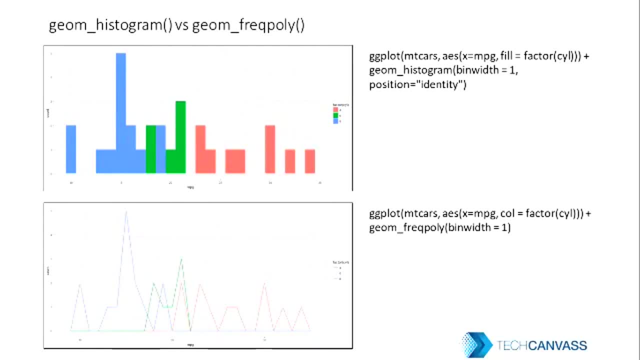 It is nothing but a replacement of histogram. Instead of bar, you can use a line or a density stuff to use The y-axis. every y-axis has a line. Every y-axis uses count. but you can also use the density on the y-axis as well. 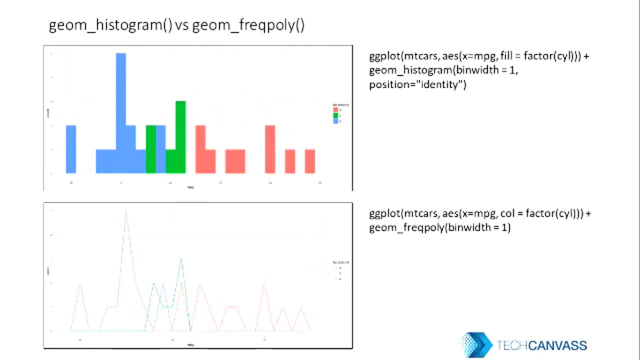 Now, what is density Instead of count? it is nothing but a cumulative percentage. You can Google yourself so that you know more about density and count. You can use free poly as a replacement of histogram if it becomes appealing to you. Next is the bar chart, the most commonly used bar chart. 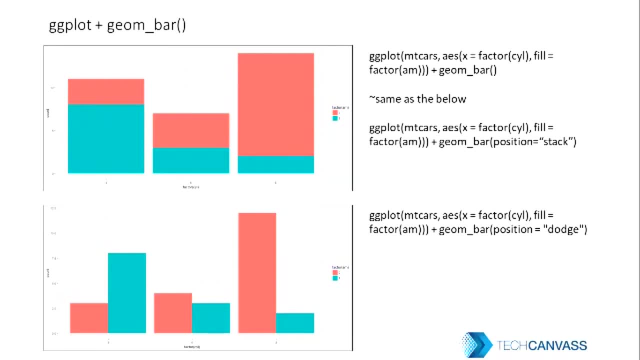 The default of ggplot is a stacking method, which you see on the first plot. The second is a dotting method. You need to explicitly mention the dotting method. Again, the structure of using geombar data- aesthetics- x-axis, y-axis- remains same across all functions. 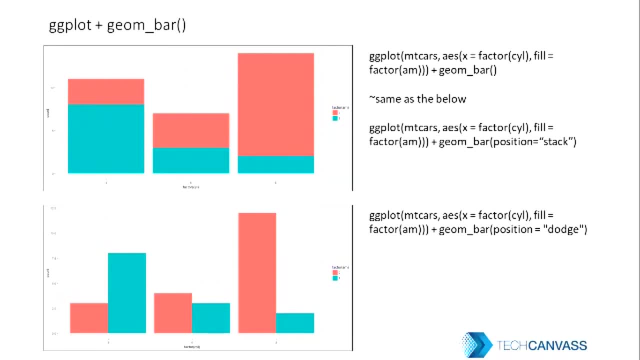 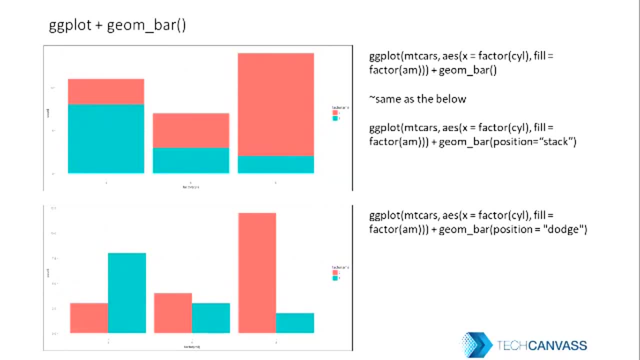 Unless you use position data. But if you are using a bar, you need to explicitly mention the position of the bar, How it will plot the bar. will it be stacked, which is by default If you don't mention anything in the first chart? 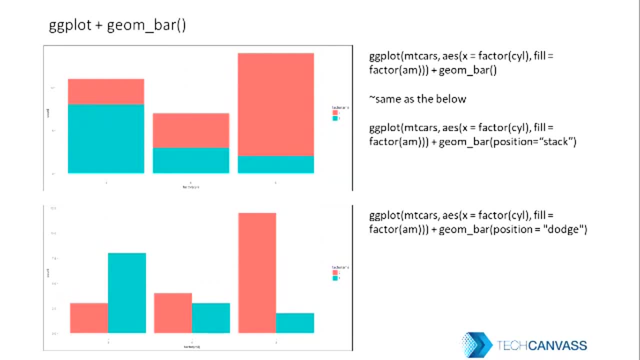 it uses a stacked chart, But if you want split charts, split bars, you need to use the dot function as well. If you mention, position is equal to dot, the plotting will happen this way, which is as traditional. Of course, you can use the stack as well in Excel. 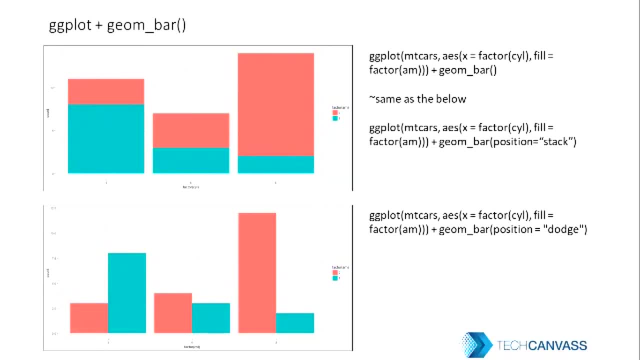 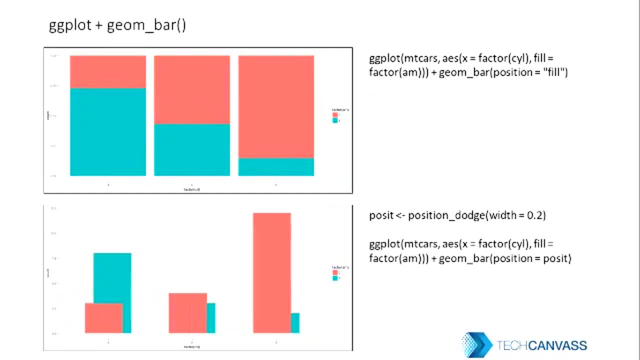 Everything you can do in Excel, but I think the default one gives a dotting method in Excel. So again, these are a few more examples. You can also position in the second plot. here You can also position the layering of the bars. 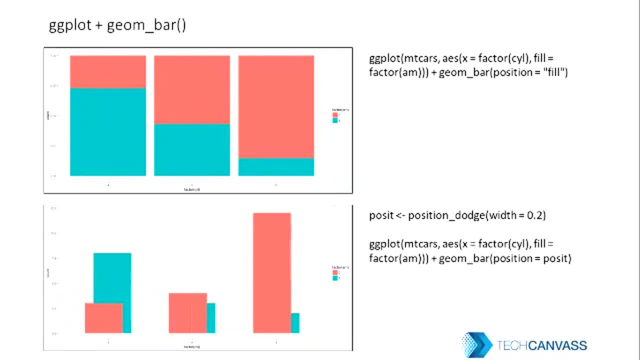 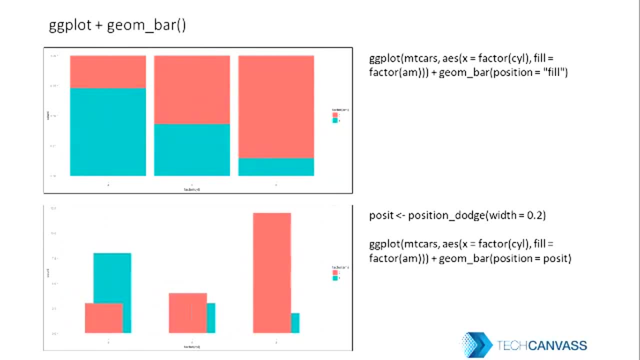 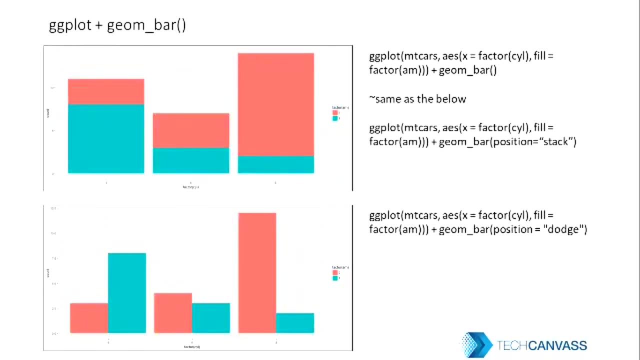 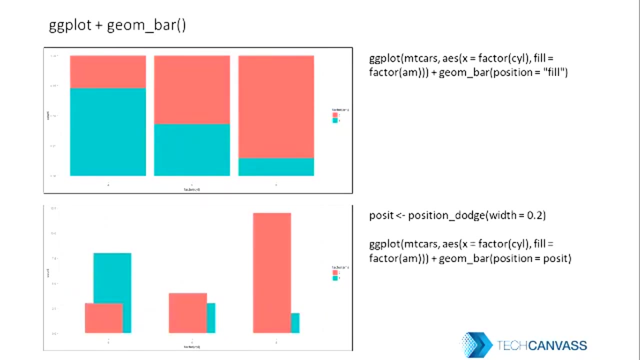 In bar you can use position Just to modify the look and feel of the bar. Just to modify the look and feel of the bar. So obviously the second plot in this chart is less attractive than the second plot in this chart. So it depends on how your taste is. 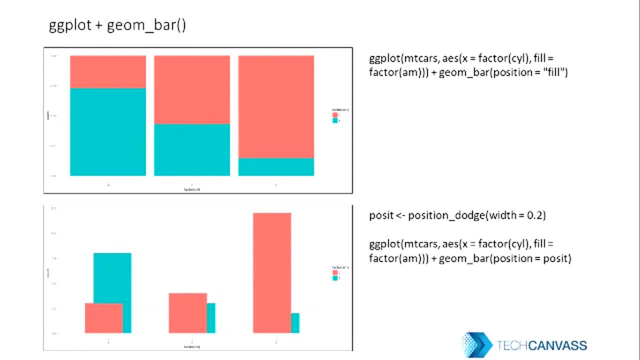 how your data is distributed. So these are all the examples. This is an example of geomline. Again, the method of using the data frame. Again, the method of using the data frame. Again, the method of using the data frame. 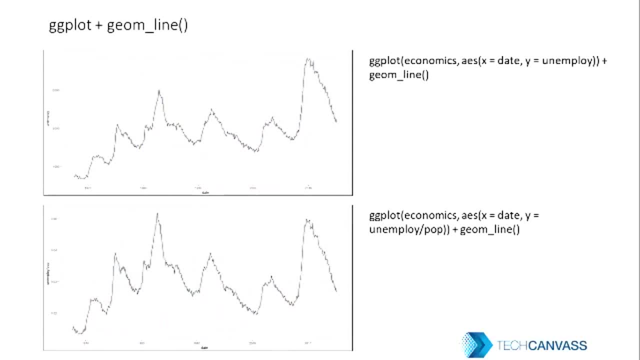 the x-axis, y-axis remains absolutely the same. No change in that. You just need to keep hovering around, whether you need a line function, whether you need a bar function, whether you need a scatterplot, what exactly you want to plot. 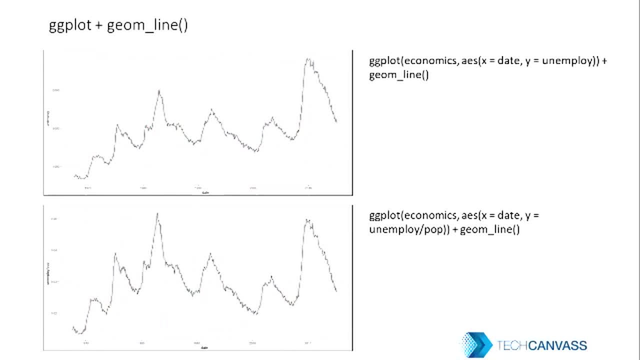 Based on that, define your function and keep plotting the data. This is way easier, way faster than the basic methods. This is way easier, way faster than the basic methods that we have around. No comparison to that. It has been tested through processing time. 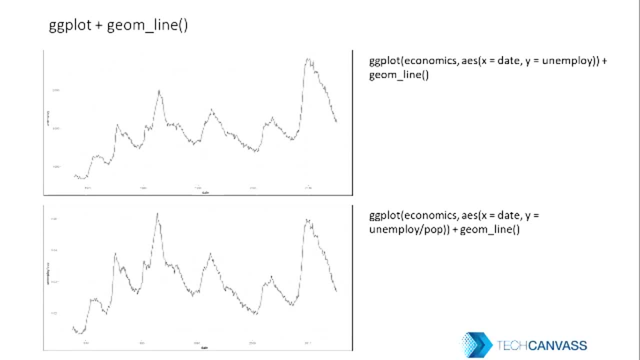 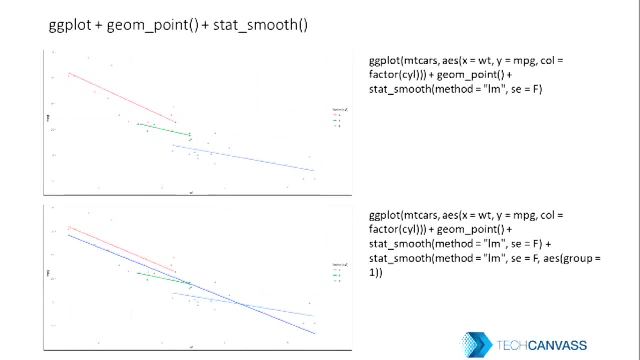 It has been tested through processing time as well as plotting time, everything way faster than the base R functions. This is again a combination of geompoint and stat smooth. You can use the coloring function as well to bifurcate the best fit regression line. 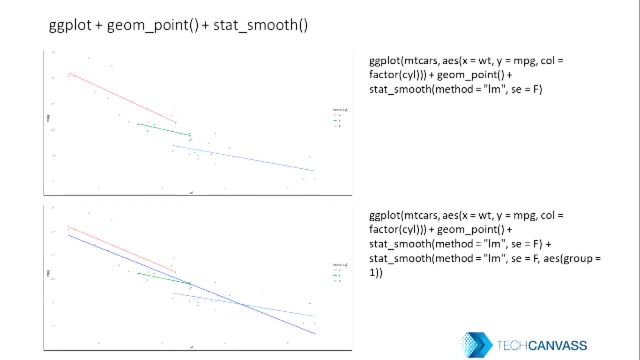 for each categories. So the first chart talks about how each category of cylinder fits in miles per gallon weight relationship, Whereas the second plot talks about definitely the individual categories but also an overall line. That's why I'm using the group is equal to one. 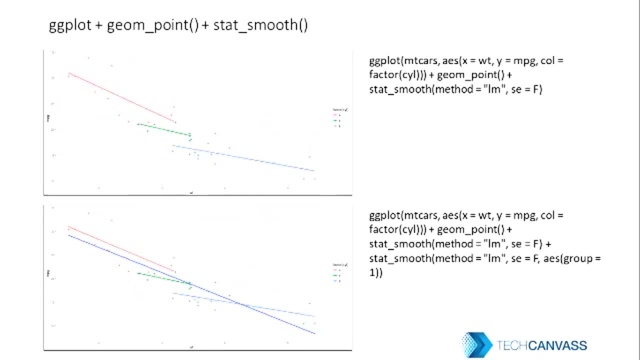 The group is equal to one, it will actually plot the overall line diagonally, The big blue line that runs across diagonally. that's, the group is equal to one. That plots the actual overall relationship, irrespective of the category's cylinder, Whereas the three plots together individual plots. 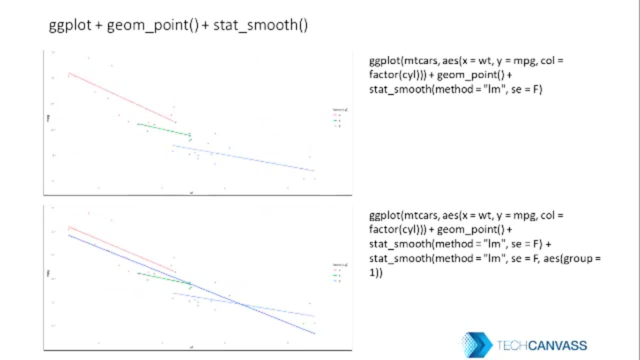 those belong to one And each plot is divided into individual cylinders. Next is the gridding system. This is very useful. You saw that in the iris dataset. But again, if you have a variable which you can AM, is a variable where I need to see the relationship. 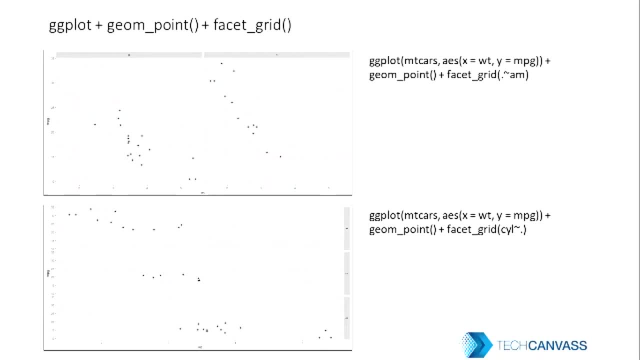 So AM goes from zero to one. So in the first chart I'm using AM, whereas it is face setting on the column wise. So dot tilde sign followed by the variable name will split the chart column wise, whereas the opposite, whereas you mentioned the variable, followed by the 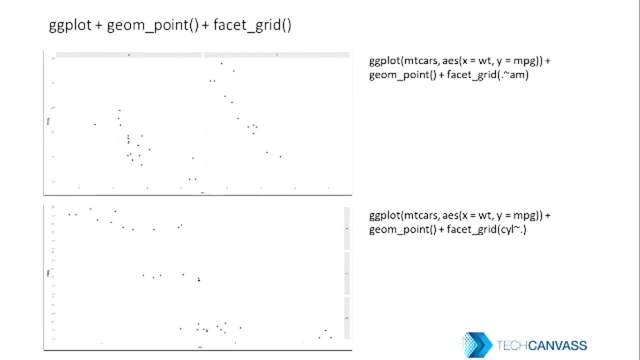 tilde and the dot sign will do the faceting robots. so, again, if you have a third variable, instead of mentioning it in the color, color argument, size argument or shape argument, if you want to do as is study, you can put them in facet. great, okay, this is a very useful tool. 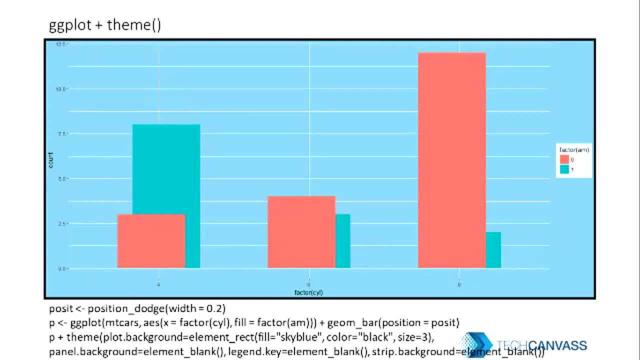 finally, the theme structure, which is nothing but the variation of how your color see the grid lines, the background color, the border lines. all those things come into the theme section. plot background, strip background, legend, panel background. everything is a part of theme. anything which is not related to the 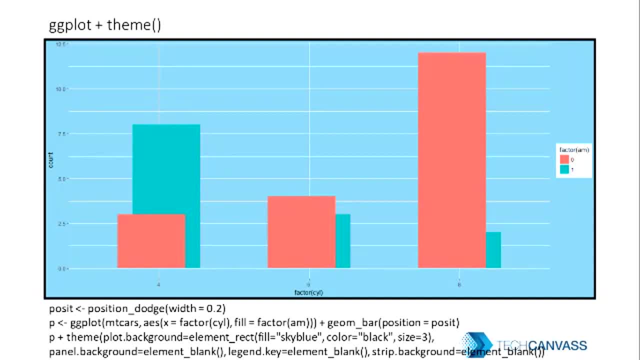 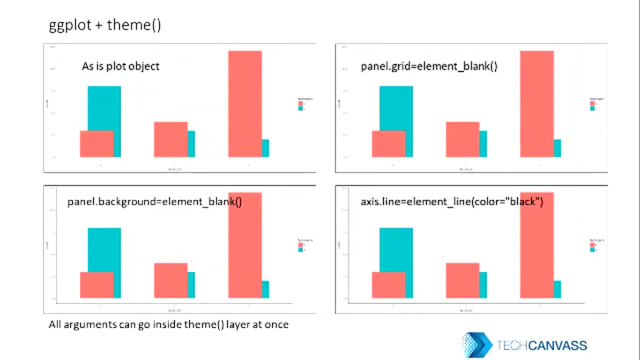 data is a part of theme. there are a lot many examples of how the theme function keeps on modifying your chart. so whatever you see here has been basically described individually in the next slides. so if you just mentioned the gg plot, followed by the theme function, the first chart, that's what you get, as is plot object. i've just picked up. 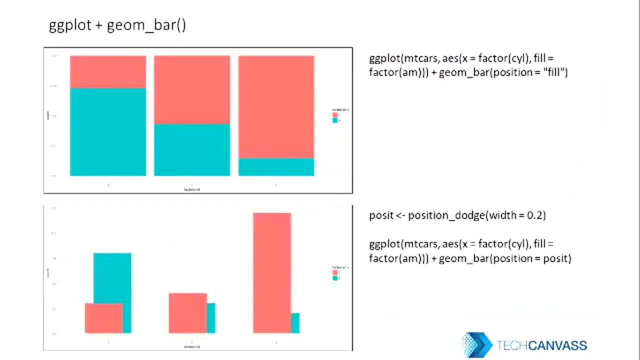 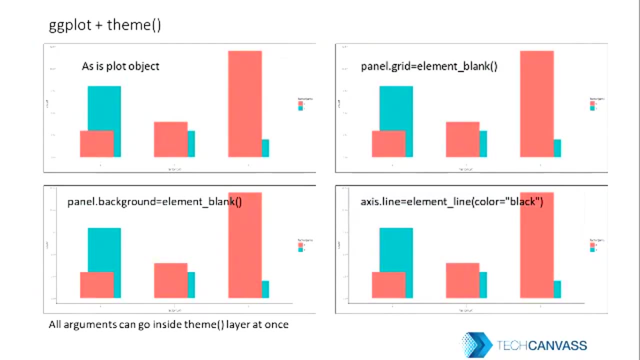 this bar chart. okay, this bar chart that you saw here. i've just picked up this bar chart. if you just mentioned the theme function, this is the as is that you get inside the theme function. you mentioned panel grid. so basically all the lines, the grid lines that you see in the panel, that disappears. 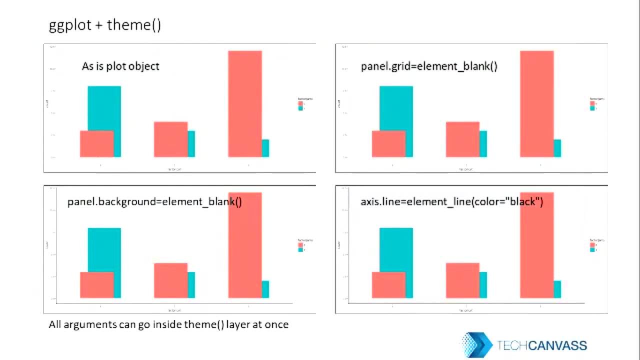 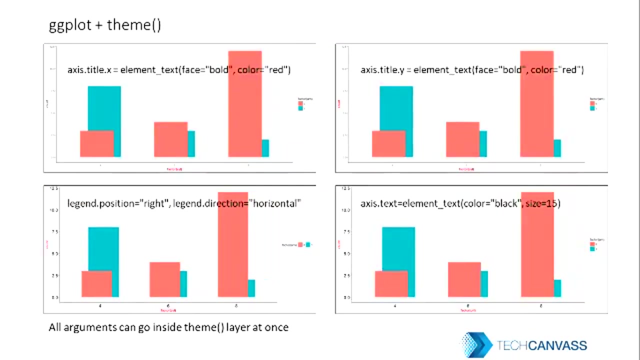 element plant means you don't want that. next, which is the third clockwise, if you mention the axis line, bold line along the axis. you mentioned the panel background, it will disappear the color that's on the background. okay, you can again keep modifying it. you mentioned the axis title, dot X. that means you want to specifically modify. 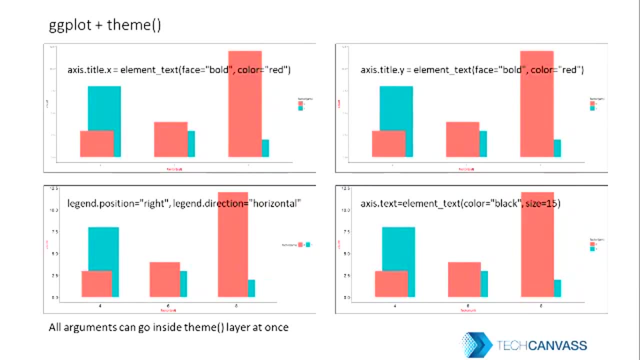 the axis title dot X. this is the piece finest part of G plot you can mention. modify each and every object that gets plotted in the job. axis dot title X becomes red, next axis dot Y becomes red and then the text becomes bold again. the actual axis structure- I mean the figures, if they are not visible- I want to make 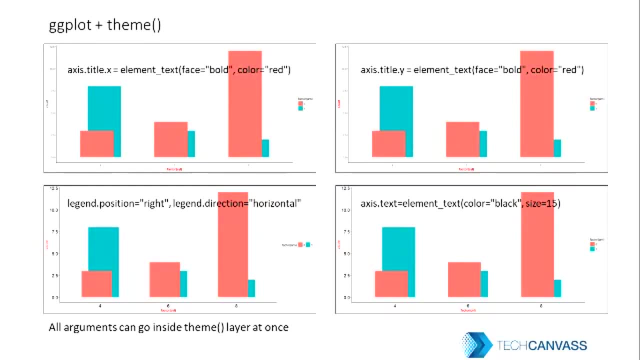 it big, I want to make it bigger. so axis dot text: put those things in element text. you know, you know. individually it sounds a little bit confusing: a lot of functions, a lot of abbreviations to remember. but once you keep doing four, five, six, eight charts, it becomes easy. okay, next is the legend. 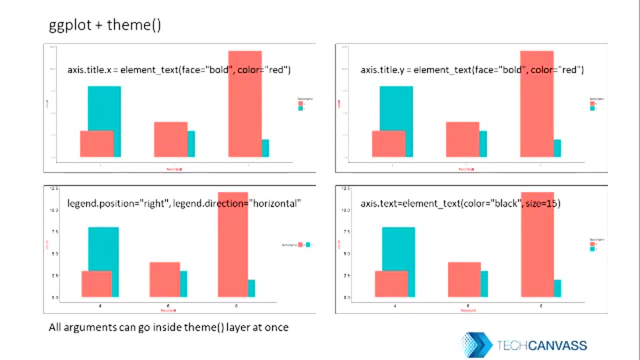 position. you can put them in horizontal or vertical method. this is, this is how you go. okay, so these are all charts, nothing to talk about. the code is mentioned in every slide, but wherever you don't see the code that's been mentioned at the notes section, keep doing. you know, please keep practicing. 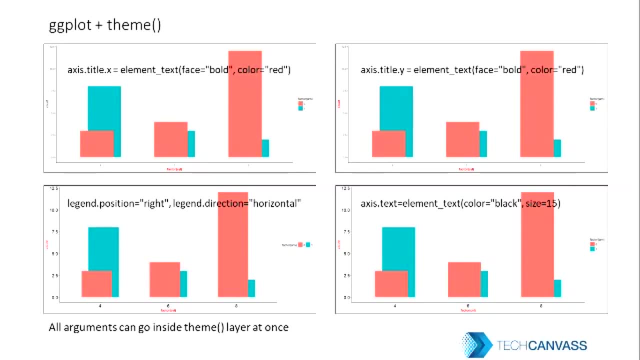 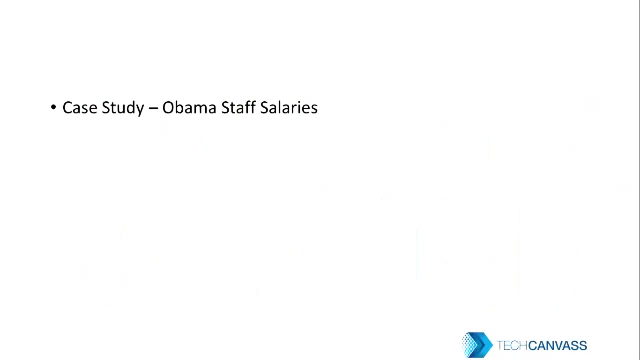 them. after you install the ggplug package. all the data sets are open. they come readily available once you install the package. nothing that you need to create, nothing that you need to modify, except the way that you want to look at it. next is: it is a Obama staff salaries data set. 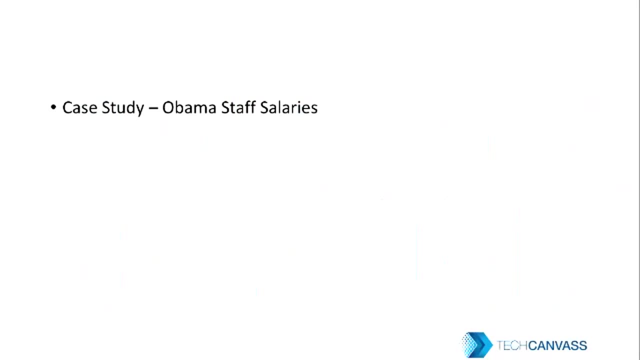 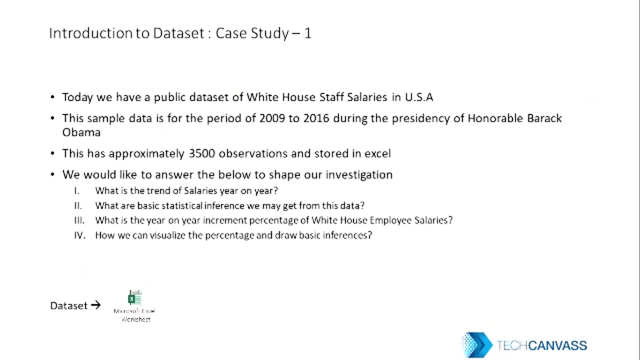 it's available in the open platform, it. this data set contains the salaries of the staff at White House during Obama's presidency. okay, so you have the data set available in Excel format. we will import the data set in Excel format. these are the questions that you want to answer from this piece. 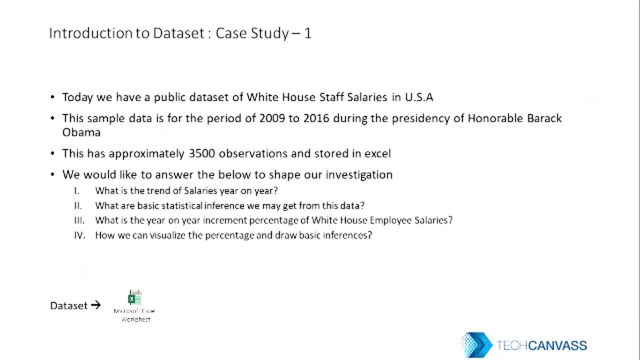 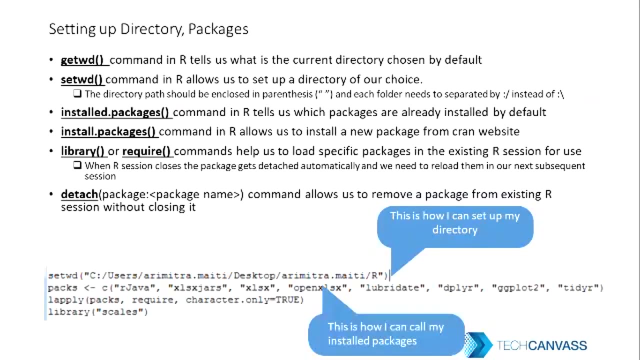 study. you know what's the trend of the salary, basic statistical inference: a year-on-year increment percentage. how can we visualize the percentage? you have the data set available. you can make your own question. you can try to answer it on your own way. so this slide talks about how you can. 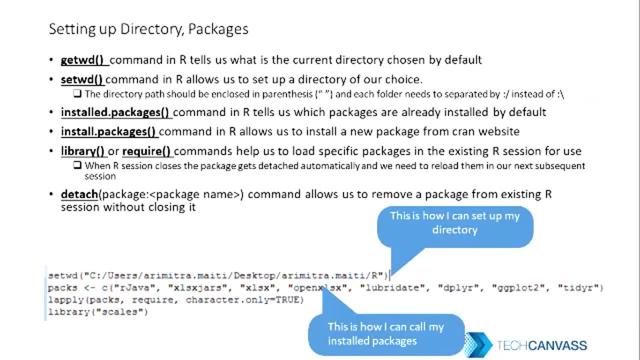 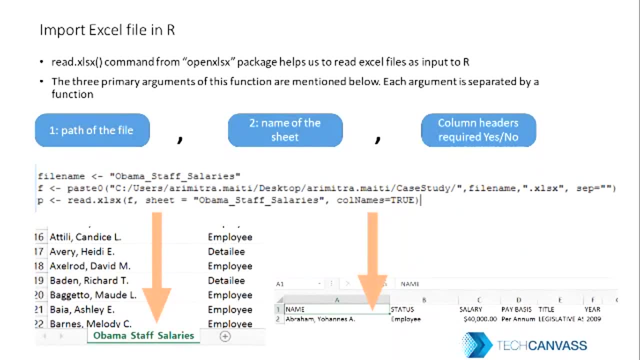 select the directory. how you install the package. this slide talks about how you use the read dot XLS X function to read the Excel data set. you just need to mention the path of the file, the name of the sheet and the column headers. this slide talks about the dimensions: how you can use the dimension, study the. 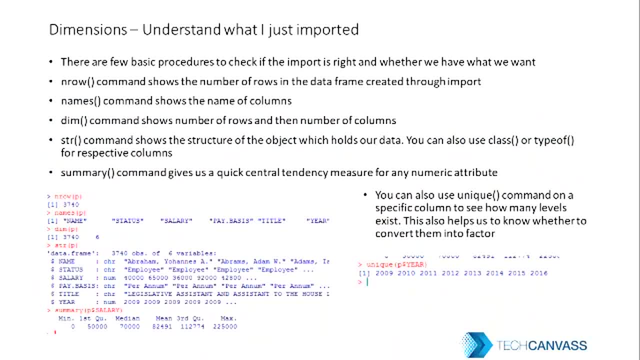 dimension. you can use the enro function, the names function, the dim function, the function to first understand what exactly has gone inside R, whether the import is successful, whether there is anything you need to modify in the import function. whether all the datasets are fine is how many missing values are. 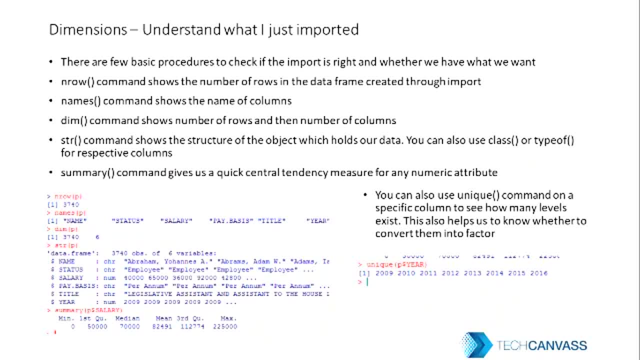 there. what's the structure of the dataset? is name a character variable? is salary a character variable or a numeric variable? what exactly you have imported? these are very good, useful function that you can use on the data sets that you have already inside the package, like empty cards. diamond either is or you can. 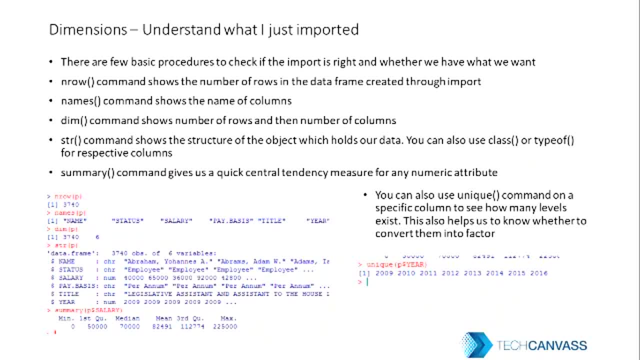 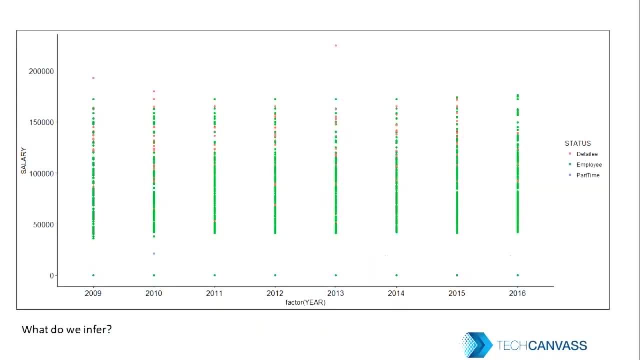 use them in your personal data sets as well. finally, this is what do we infer from the chart. the code goes is mentioned in the notes section. so you can see that, you can see that. so you can see that. so you can see that the green color is of employee, the red color is of detail and the blue color is. 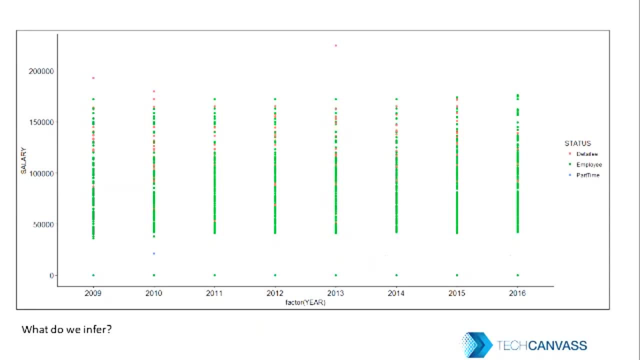 of a part-time category. so there are three categories of employees that we can see we have in the data. okay, detailly employee, part-time. the number of employees are obviously very distinctively higher than detailly and part-time. obviously part-time make sense, but detailly I think they are more. 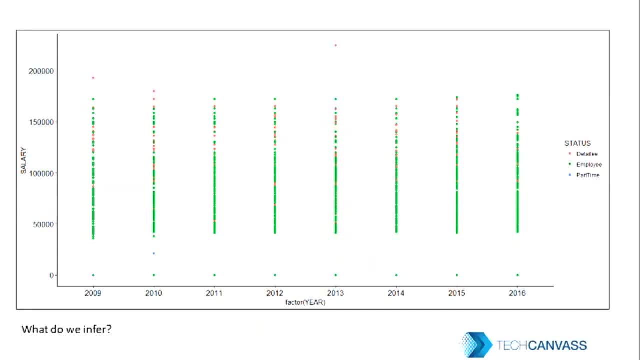 expert. why they are more expert? because you can see that every year the salary of detailly is way higher than the employees. okay, so obviously we can infer that detailly are more expert people. they give specialized- you know, they do specialized jobs compared to employees. basically, you know, the regular employees. 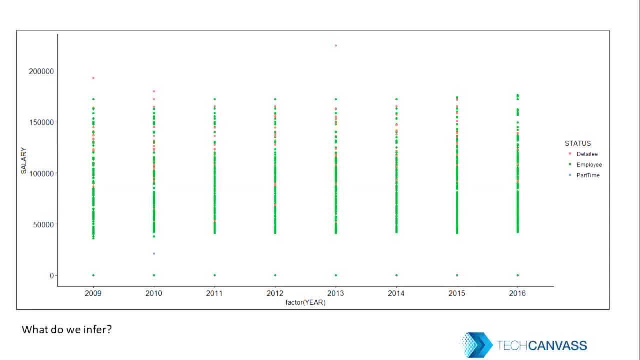 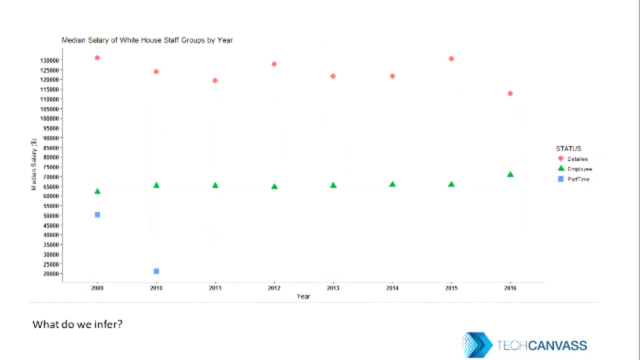 and obviously the salary of employees ranges from high to low. okay, the y-axis is the year, the y, sorry. the y-axis is the salary. x-axis is the year. finally, I want to know the median salary of each group. so every data y axis is a year, so I take that back. the y-axis is the median salary, the x-axis 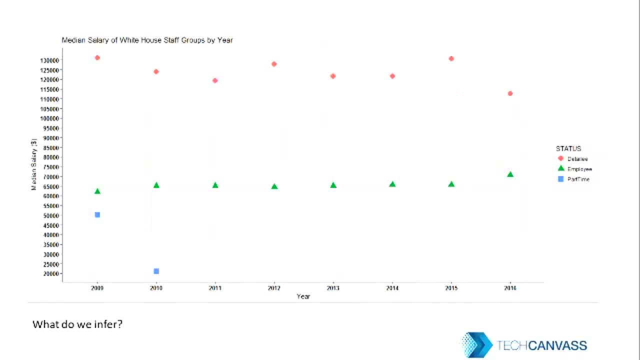 is the year and each color is the color of status. so you can see that our influence was right, that median salary of detailly is way higher than the employee of the part-time, whereas the median salary of employee is way higher than the part-time. this is how it goes on increasing first part-time. 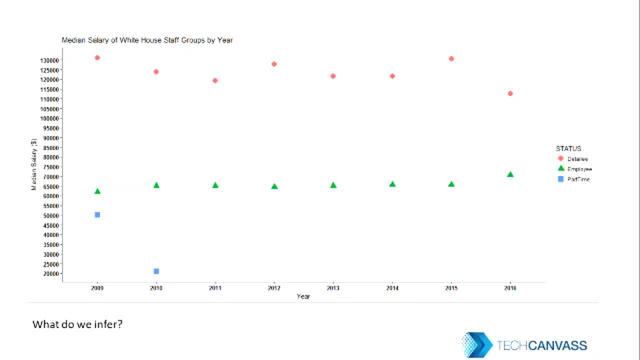 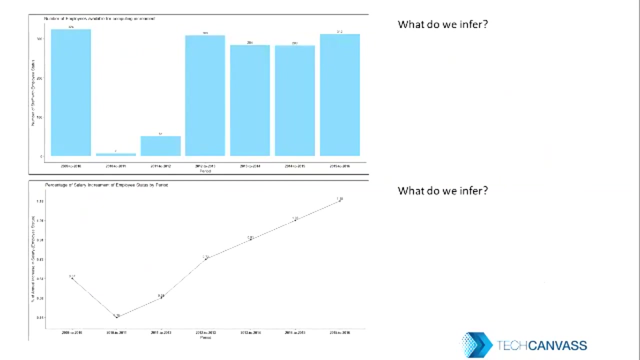 employee and, detailly, should be more experienced and specialized in their jobs. okay, so this is one influence we can get. next, I wanted to ask whether we can calculate the increment percentage of salaries for, specifically to employees, the green in color. so what I did is I ran a piece of 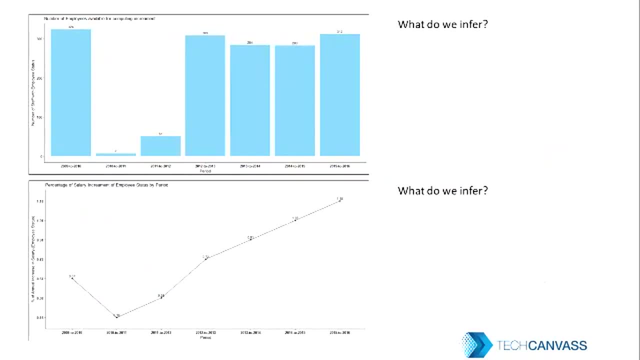 code wherein I calculated how many number of employees we have from year to year. so we can see: from 2009 to 2010 we have 324 employees which qualify for an increment. so those employees were there in 2009 as well as 2010. otherwise, I. 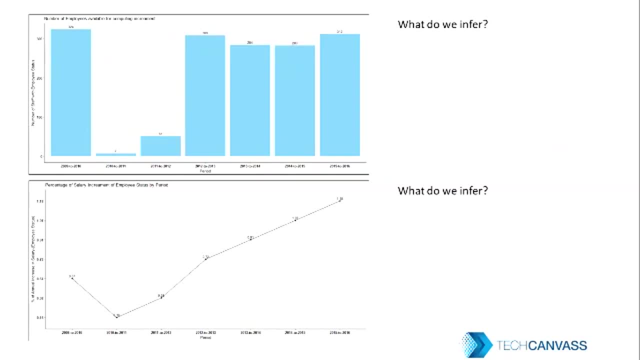 cannot count, Calculate the increment right. same goes for 2010 to 11,, but I have very low number of people in the data set, whereas in 2015 to 16- same people, There are 312 people who got the increment. Okay, so what's the? 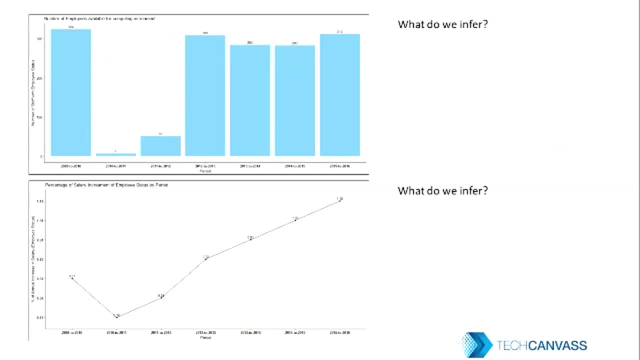 actual increment rate. Okay, percentage of annual increase in seven. so I can see that 2009, Because you know, around zero points, six, seven, whereas it we move to around more than hundred percent, 2015-16. so the increment percentage is Kept on increasing, although we see a dip in 2010-11, which is point one, five. 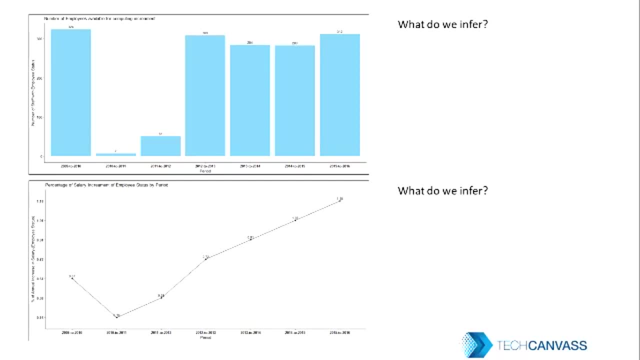 But I think that's a bad data point. We can't compare the increment based on only seven employees. We would actually need a minimum of 30 employees to calculate anything which we have 2011-12. we have more than 30, 51 and the percentage is 0.39. 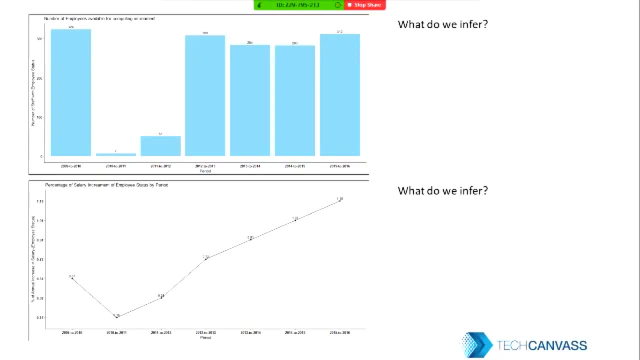 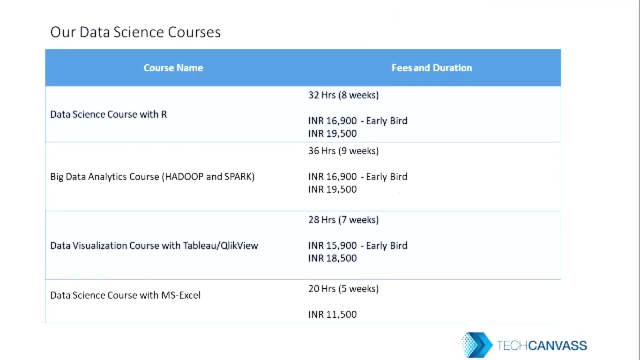 So, except 2010-11, I think, the percentage of annual increment kept on increasing. So This is the final slide at tech canvas. These are the different categories of courses. We have a data science course with our 32 hours, big data analytics course for Hadoop and spark. 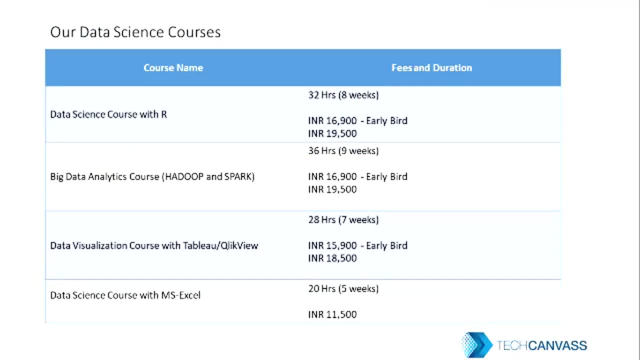 That's for 36 hours. Data visualization course with tableau and click you especially, that's for 28 hours. Data science course with MS Excel: That's for 20 hours. We do have an early bird discount for data science course, especially with revolution. are please do? 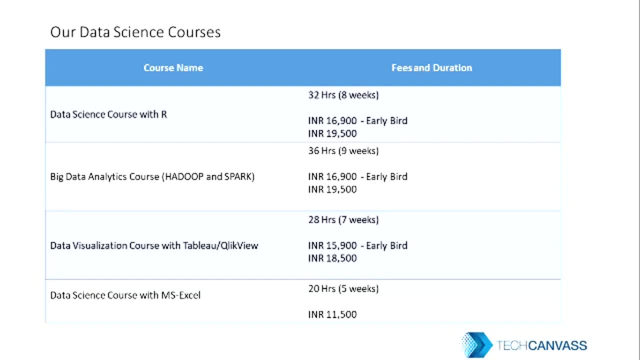 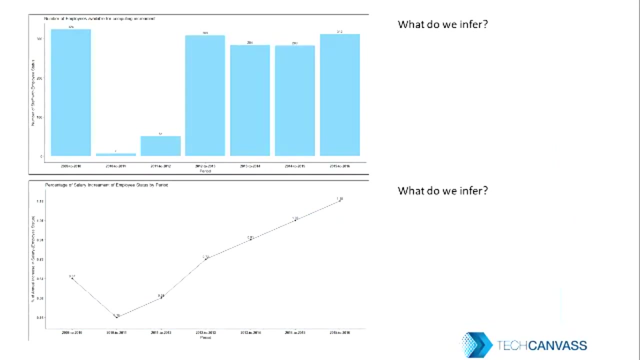 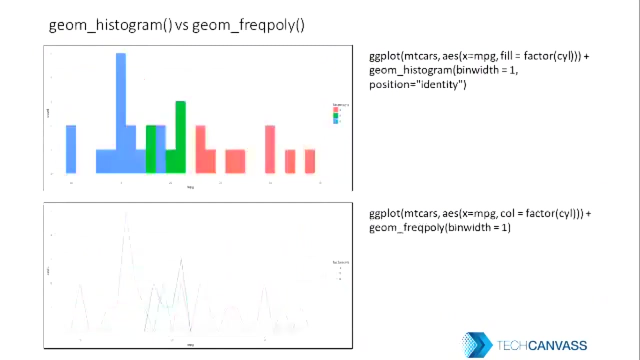 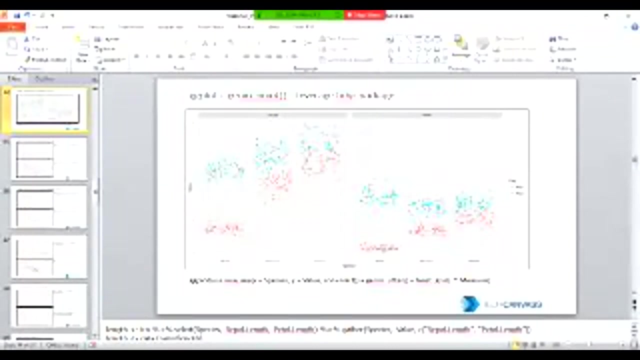 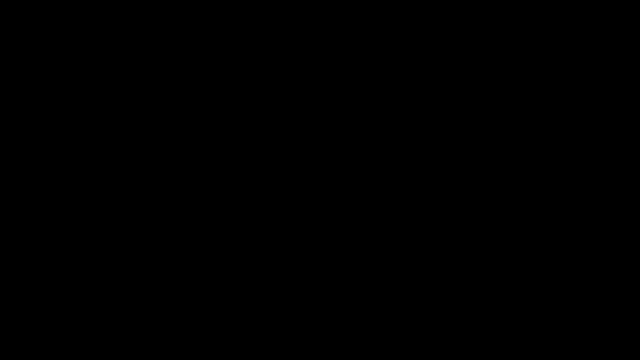 Keep in touch with Nazni or the campus office so that you can pay this discount. I Still have 25 minutes of today's discussion. I Leave it on to the audience So that they can ask their doubts. You, if you have any question, please go ahead and ask. I see on the. 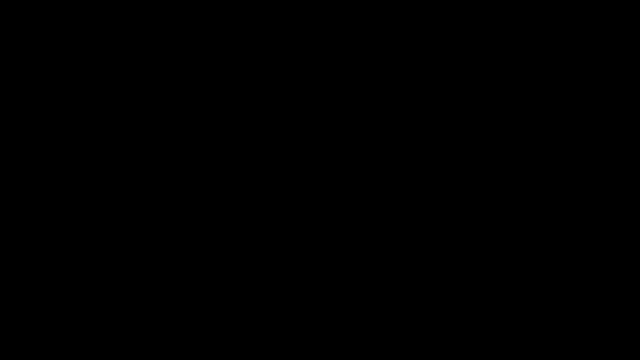 two parts best race mine so needing. so if you do have Question, please go ahead and ask, Or else you have the material available. with nasty or she wonky You can take that material, install our, install GG package and keep practicing. You, You, You, You, You You. 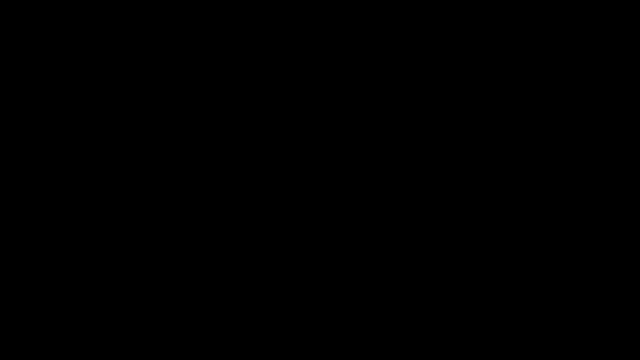 You? okay, shall I assume that we don't have any questions so far? Reshma, she won Sunni. okay, Sunni lying here from Reshma as well. I mean, if you don't have a mic you can type. if you don't have any question and if you are interested in this topic of 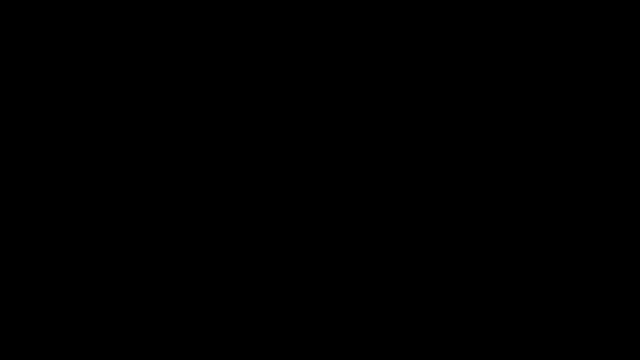 ggplot. please do take the material from the canvas and ensure you do come back if you have any question. all the basic stuff has been already put. oh, thank you, it was quick, I think. so there are no questions. so any query apart from this? we have a contact number.